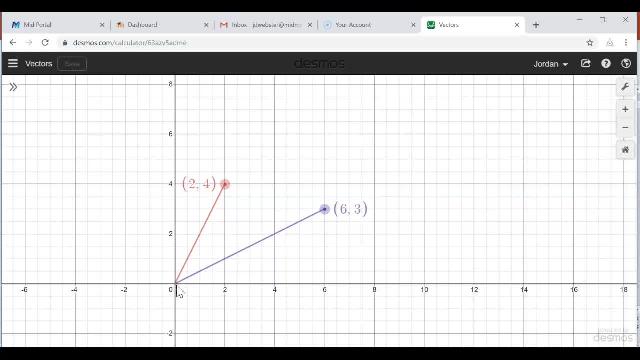 And basically what they are is the line segment. you can think, from the origin to the point 6, 3, or the line segment from the origin to the point 2, 4.. Okay, And no matter where we put this, vectors are always going to have some sort of an x-value length. 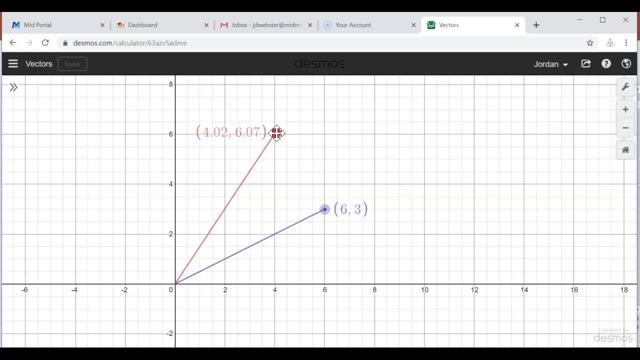 some sort of a y-value length. Now, this is in two dimensions. In three dimensions we would go out to we'd have an x, a, y and a z. So vectors are in some ways equivalent to the idea of. 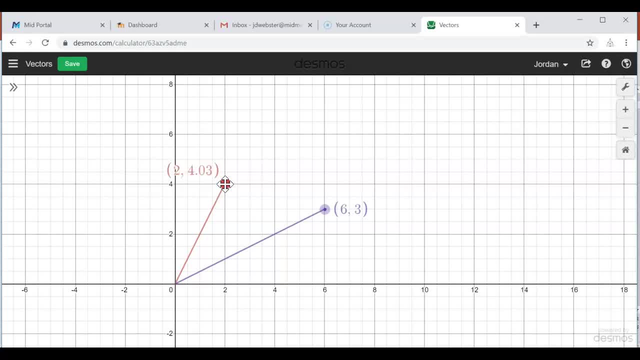 hmm, let me get that stick it for sorry. there we go of the points where they end at right. So we're going to look at a couple of different ideas of vectors, and I may refer back to this slide to see what's happening. 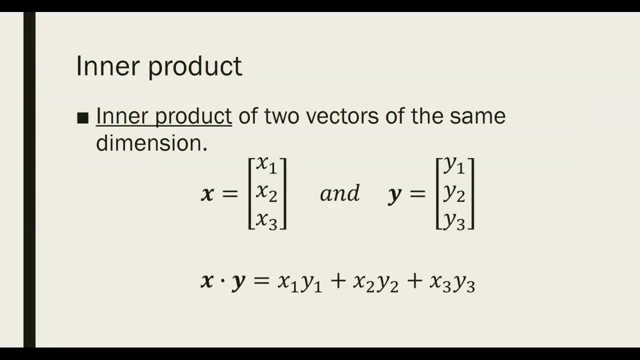 All right, So let's start with interpolation. Now. we all know that we can't multiply two vectors together under normal matrix multiplication operations. However, there are a couple of different ways in which we can define multiplication of two vectors Now. one of those is called the inner product. 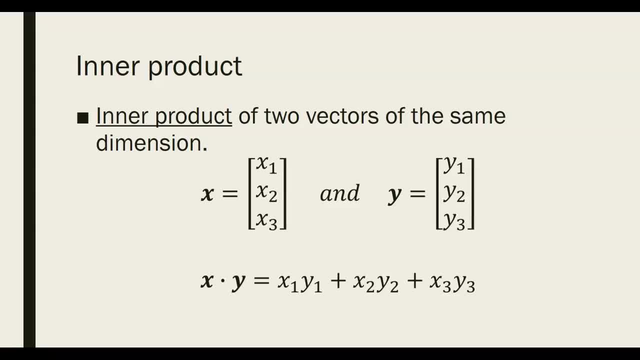 Okay, Now, in order to calculate an inner product, the vectors have to be of the same dimension, So, like in our case, in front of us we have three-dimensional vectors. They come from R3. And the inner product of two vectors is always going to be written as: vector x dot vector y. 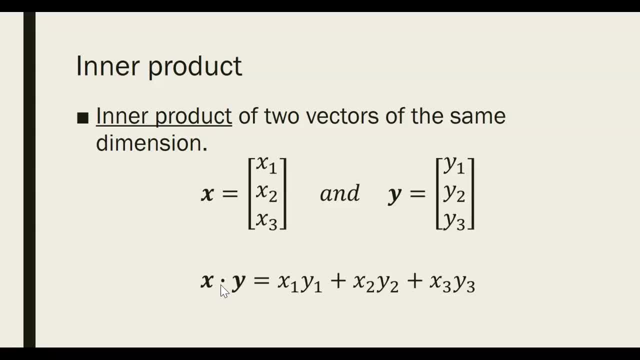 Okay, So this is the standard notation for inner product. There's a dot there. By the way, there's also something called a cross product that we're not going to look at in this section, But cross product comes up when you deal with topics in Calc 3,. 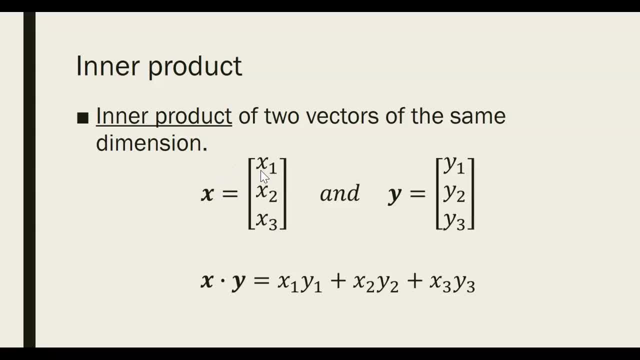 Most things Now notice what the inner product is doing. We're taking the first entry of our vector x and our first entry of our vector y- Okay, y- and we're multiplying them together, And then we're taking our second entry of x and our second. 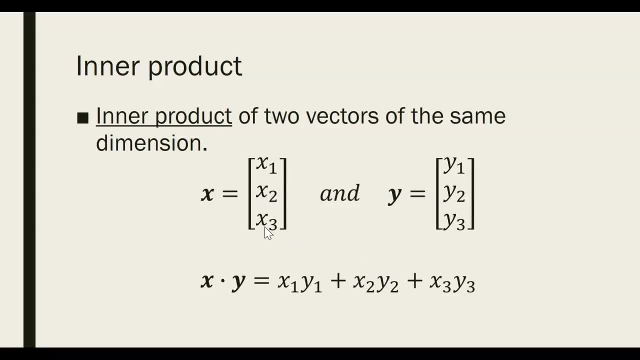 entry of y, multiplying them together. Our third entry of x. third entry of y, multiplying it together and then adding them all up. So notice that when you take an inner product of two vectors, my answer is going to be a real number, at least as long as the entries are real numbers. 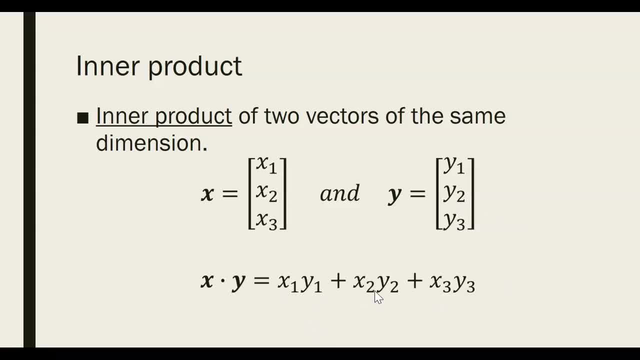 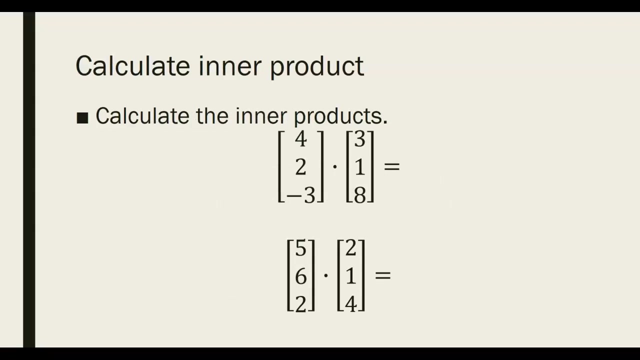 So if I have real numbers that are multiplying and adding together, we're going to get real numbers. So I took two vectors from R3, and I ended up with a real number answer for my inner product. So I want you to push pause on the video and try to calculate inner products. 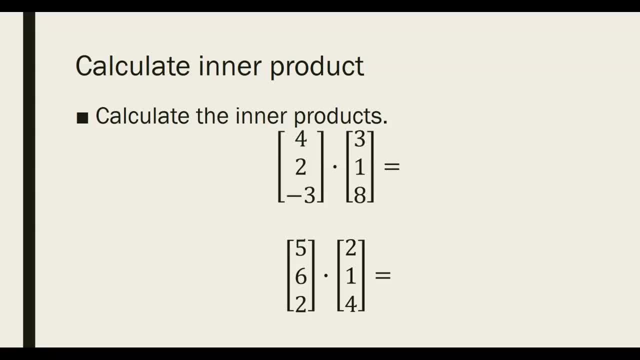 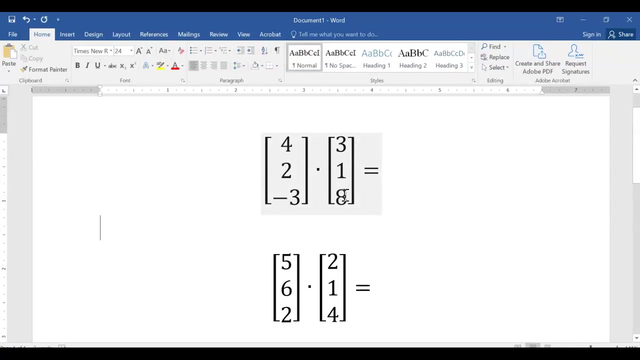 of these two examples. So we have two vectors. we're taking inner products of. Again, notice the notation. The notation we use is a dot when we deal with inner product. So go ahead and push pause and do that, Okay. so let's go ahead and do that. So I'm going to take the inner product of 4, 2, negative 3, with 3, 1, 8.. 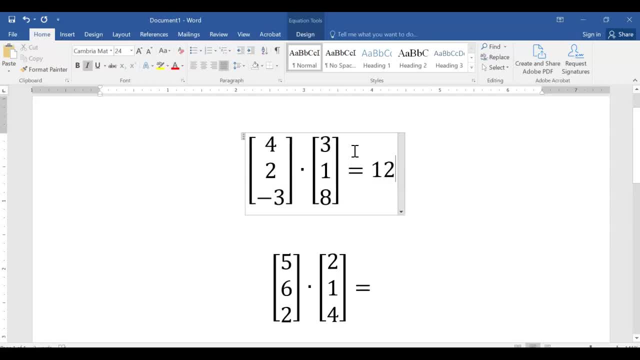 So all I do is take 4 times 3,, which is 12,, plus 2 times 1,, which is 2,, plus negative 3 times 8,, which is negative 24.. Whoops, And so the inner product of those. 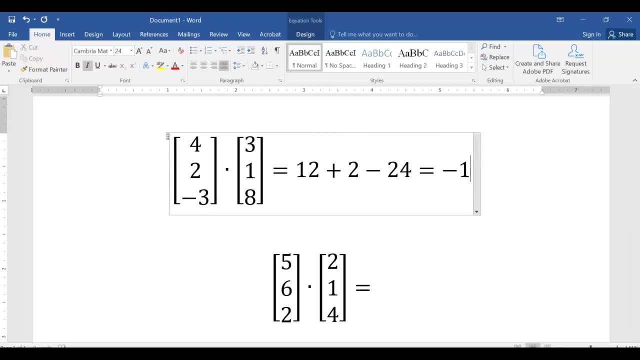 two vectors is going to be negative: 10.. Alright, These next two vectors: 5 times 2 is 10,, 6 times 1 is 6, 2 times 4 is 8.. So the inner product of those two vectors is 24.. 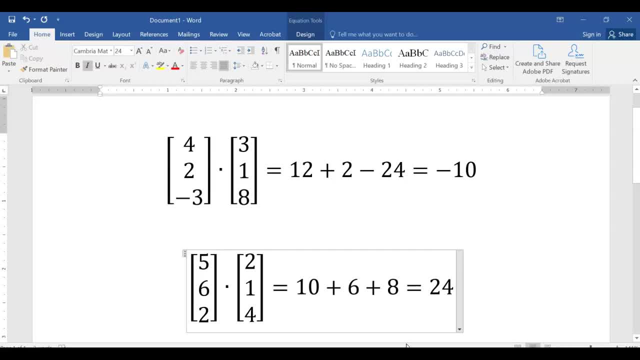 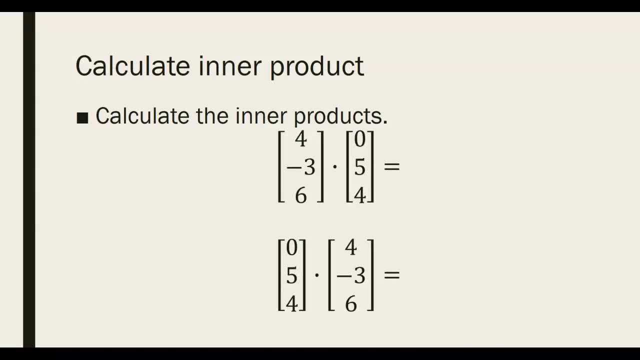 And that's it. That's the inner product. I want you to now calculate the inner product of these two vectors, making note of the fact that these two vectors- 4, negative, 3, 6,- I've put on the left-hand side in my first multiplication and the right-hand side in my second multiplication, and 0, 5, 4, I've put on the right-hand side in my first multiplication and 0, 5, 4, I've put on the right-hand side in my second multiplication, and 0, 5, 4, I've put on the right-hand side in my first multiplication, and 0, 5, 4, I've put on the right-hand side in my second multiplication, and 0, 5, 4, I've put on the right-hand side in my first multiplication, and 0, 5, 4, I've put on the right-hand side in my second multiplication, and 0, 5, 4, I've put on the right-hand side in my first multiplication, and 0, 5, 4, I've put on the right-hand side in my 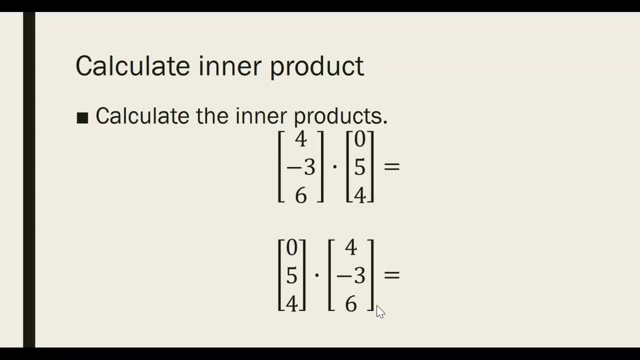 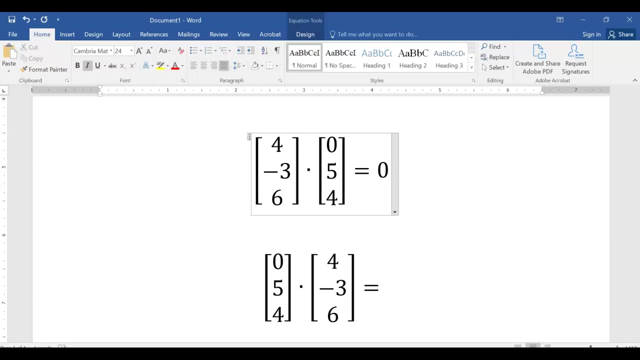 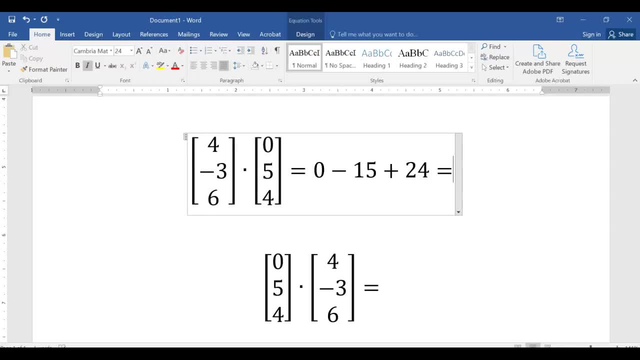 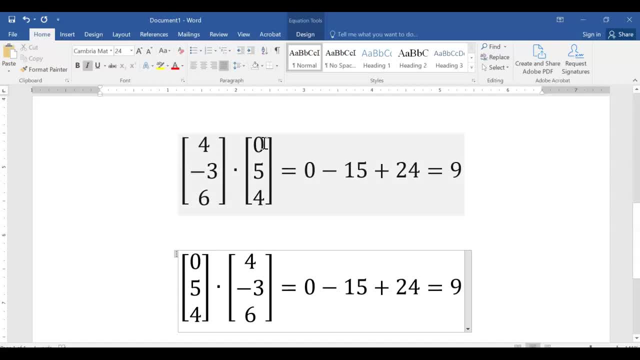 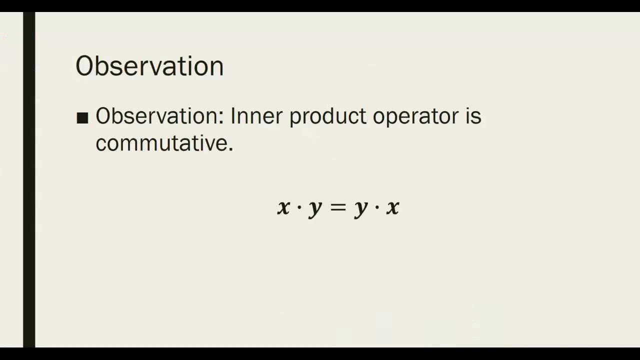 explanation, You get the same thing in each one, because obviously when you multiply two real numbers, that multiplication is commutative. So what this tells us is that the inner product must also in fact be commutative. So that's the observation that we see there. So the inner product as an operator is a commutative operator. So if you can take the inner product of 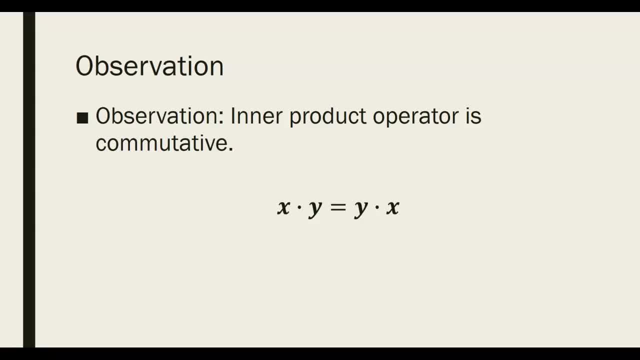 x times y or x dot y, then you're going to get the same thing as y dot x. Now there are some other properties of inner product. I'm not going to demonstrate these, but it turns out when you take three vectors. 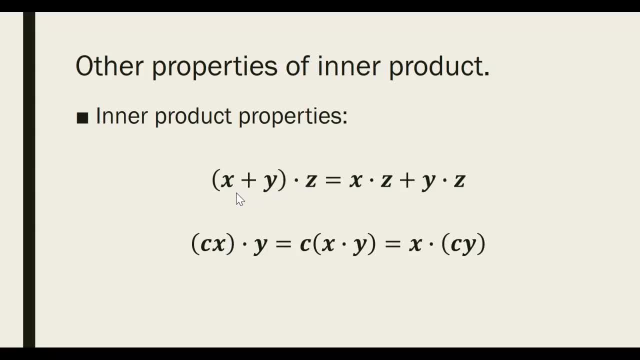 x, y and z. if I want to add x, y and then take the inner product of that with z, you could have sort of distributed the inner product multiplication into both the x and the y, And inner product is commutative, so we could have, you know, commutatively done that as well. 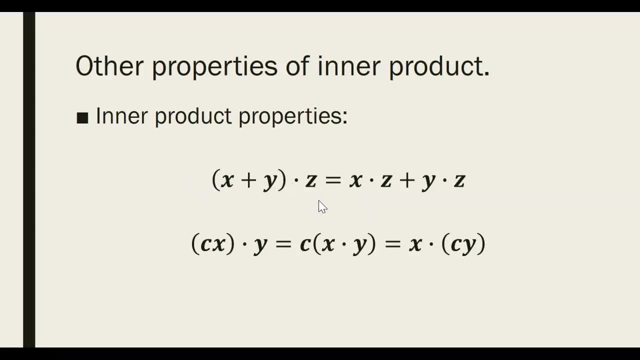 In other words, we could have put the z on the left-hand side or the z on the right-hand side, So inner product distributes over addition. And then the other little fact about inner products is that they work well with constant numbers. 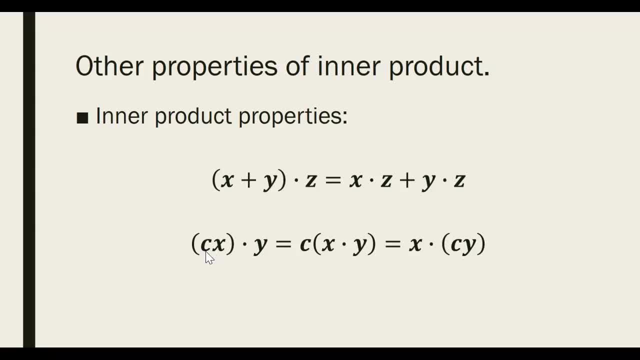 So if I take a constant times x- again, that's little c stands for any real number constant here- and then do an inner product with y. well, you could have done the x inner product, y, then multiplied by the constant. 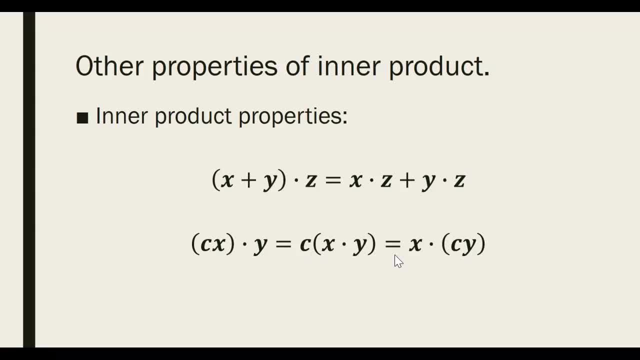 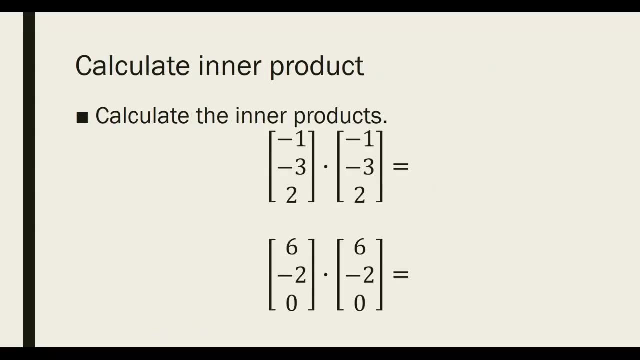 or you could have multiplied by the constant times y, and then did the inner product with x. So constants can kind of distribute in and out of the inner product as we would like. Now I want you to take a look at the inner product of a vector with itself. 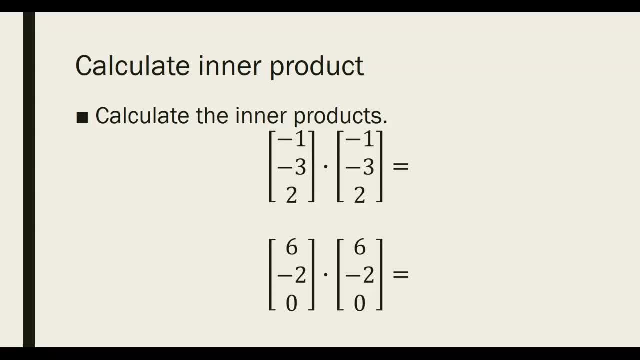 Okay, So let's take the inner product of negative 1, negative 3, 2, with itself and the inner product of 6, negative 2, 0, with itself. Go ahead and push pause on the video. 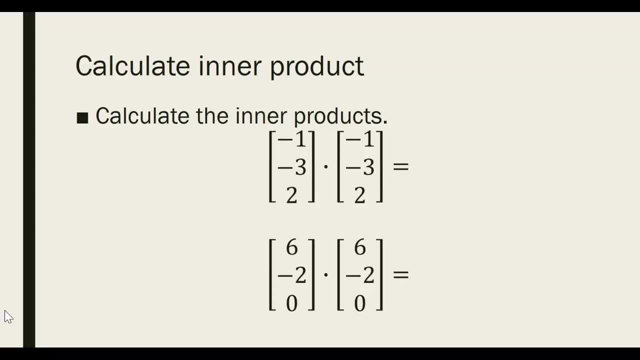 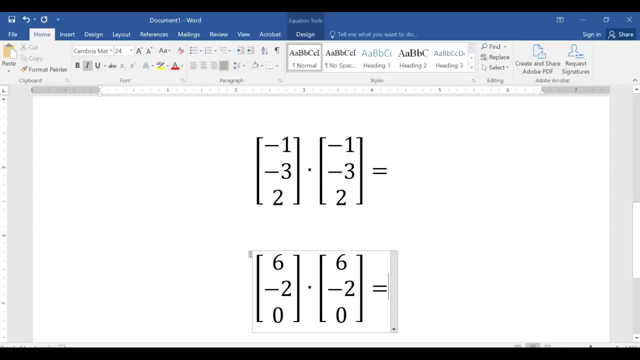 and calculate this, these inner products. Alright, so here we go. Negative 1, negative 3, 2, and 6, negative 2, 0,, each multiplied by themselves in terms of inner product multiplication. So negative 1 times negative 1 is a positive 1.. 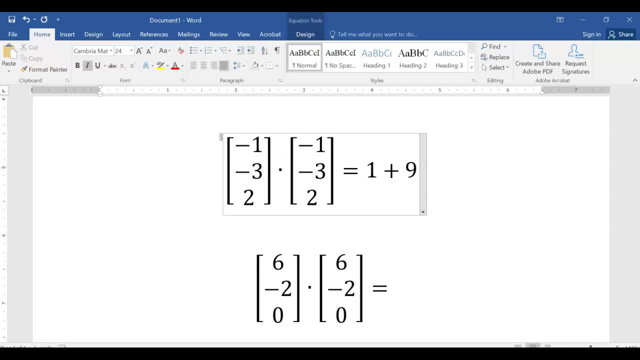 Negative 3 times negative, 3 is a positive, 9.. Negative 2 times negative, 2 is a positive, 4.. So when you add up all those things, you get a 14.. When I take a 6 times 6, gives you 36.. 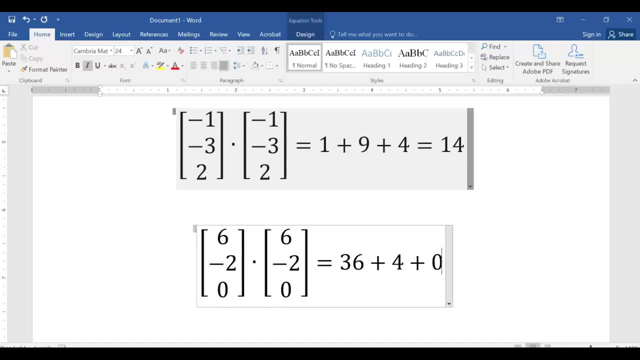 Negative 2 times negative. 2 gives me a positive 4, and then plus 0. So you get a 40.. Now what I want you to observe is that when you take each entry and you add up all those things, you get a 14.. 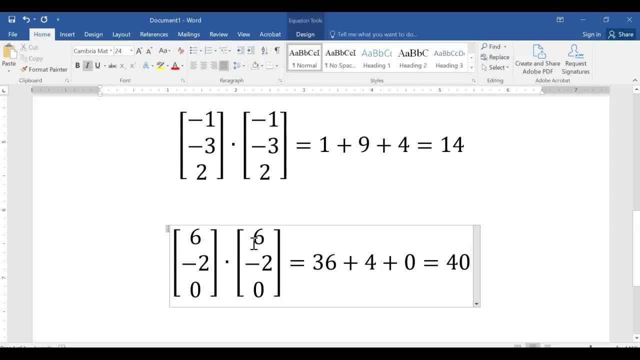 So what I want you to observe is that when you take each entry times itself, it's basically that entry squared. So notice that all of these things you add up are going to be well positive or 0. So we say non-negative. 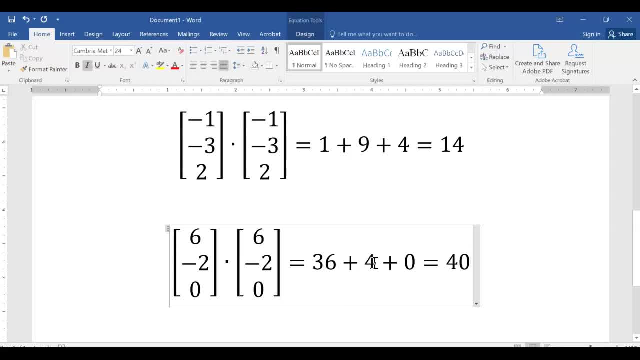 So we're never going to get any negatives when we do the inner product with a vector by itself, And the only times that we get 0 is when it's 0 times 0. Okay, And if we do the inner product with a vector by itself? 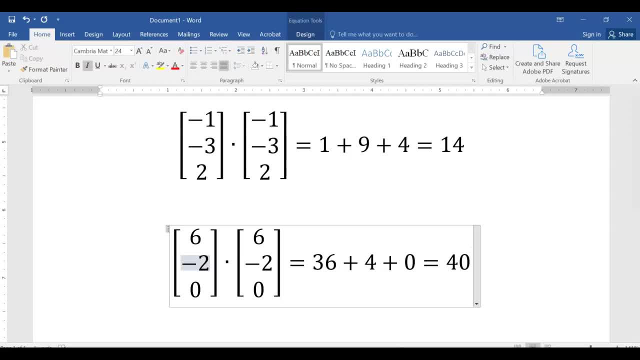 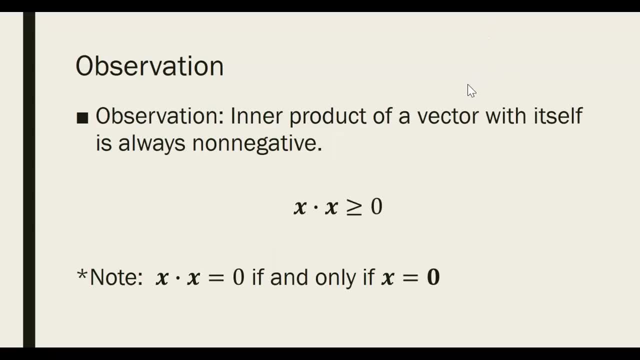 if you think about it, the only way you can get a 0 as an inner product is if we have the 0 vector. So in other words, the inner product of a vector in itself is always going to be non-negative, because when I take, the inner product of a vector times itself. 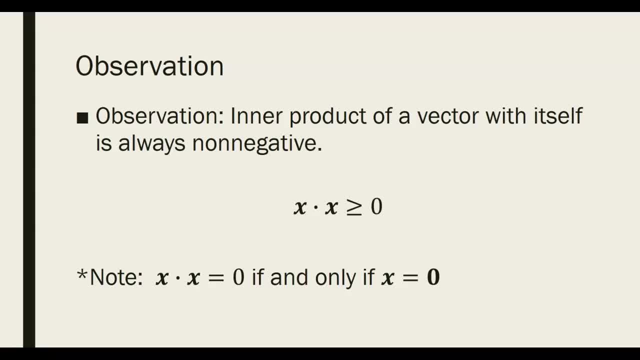 I'm basically squaring each entry of the vectors and then adding them all up, And the only way- the only way you can actually get out a 0 is if we start with the 0 vector. So there we go. Now, this is nice because of what we're going to look at next. 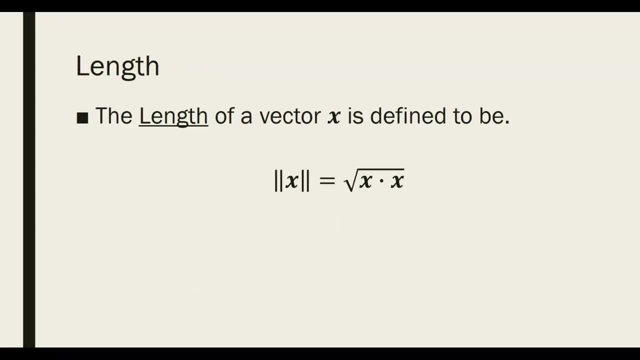 We're going to look at the length of a vector And we're going to define the length of a vector to be the sum of the length of a vector. So we're going to take the square root of the inner product. So again, the inner product is going to be a real number. 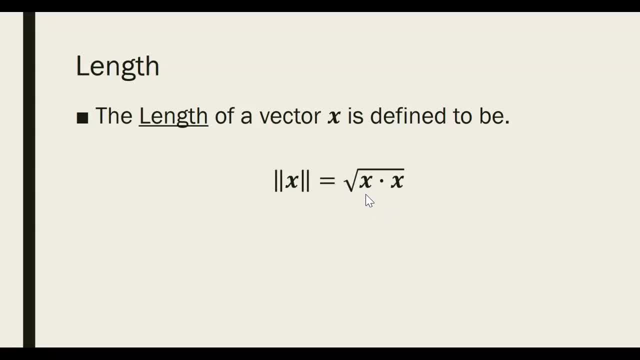 and we're just going to take the square root of that. We just saw that this is going to be non-negative, so it should be always possible to take a square root of it. as long as our vector x has real number entries, Alright. 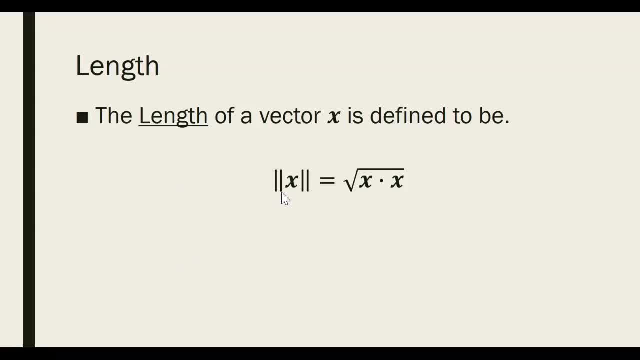 And, by the way, the number entries are going to be real numbers, So the notation of length of a vector is going to be: it kind of looks like two absolute values inside of each other, So it's two vertical bars on the left of the vector. 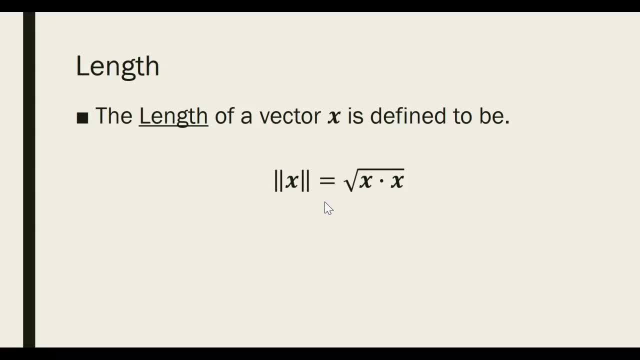 two vertical bars on the right. So inner product is the square. excuse me, length is the square root of the inner product. So let's go ahead and calculate length of these four vectors. Push pause on the video. do the square root of the inner product? 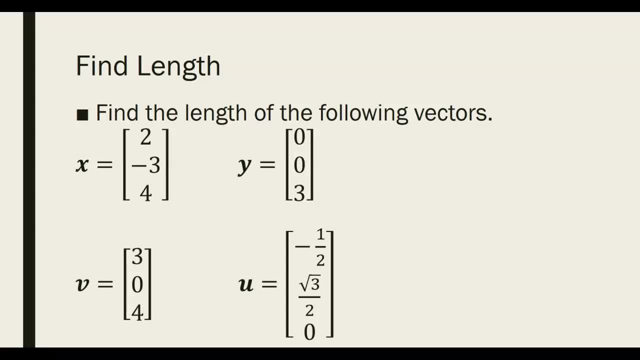 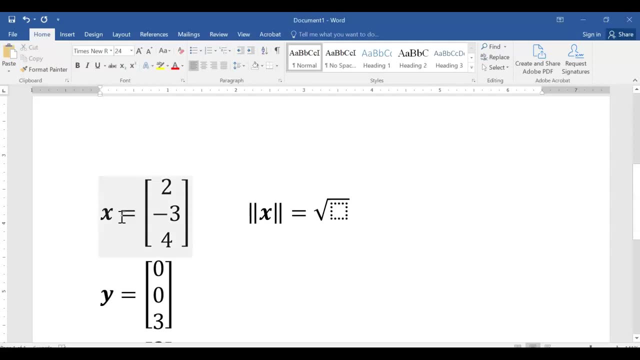 with the vector times itself and figure out the length of these four vectors. Alright, so here we go. Let's take the length of. so we're going to take the inner product of x times x. So what that's going to do. 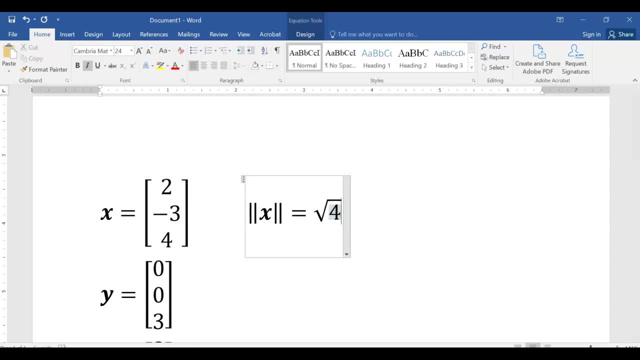 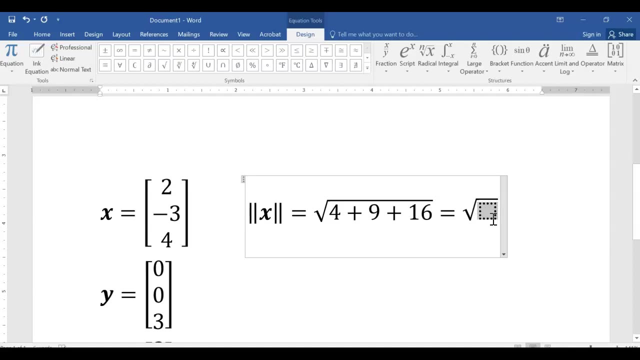 is it's going to do 2 times 2,, which is 4, plus negative 3 times negative, 3,, which is 9, plus 4 times 4,, which is 16,, which gives you the square root of, I believe, 29.. 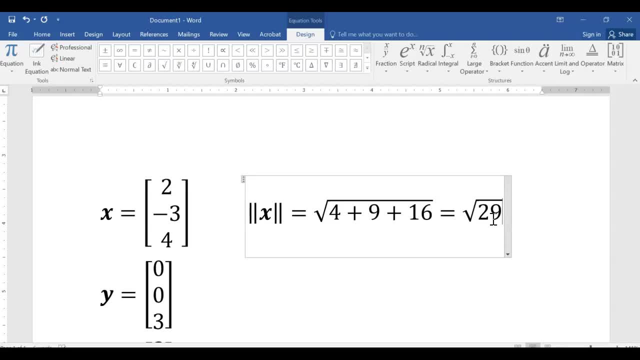 Okay, So let me double check that: Yep 29.. And that's it. Now, if you wanted to round the square root of 29 or simplify the square root of 29,, by all means go ahead If you wanted to, you know. 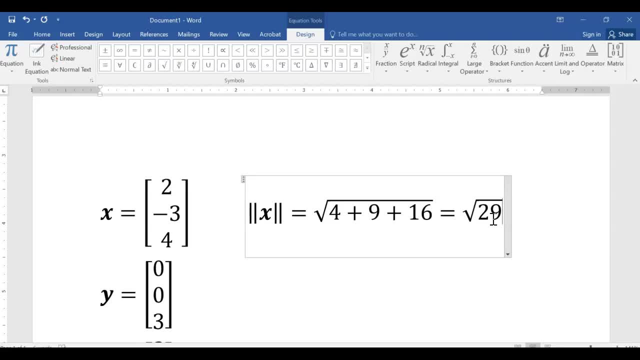 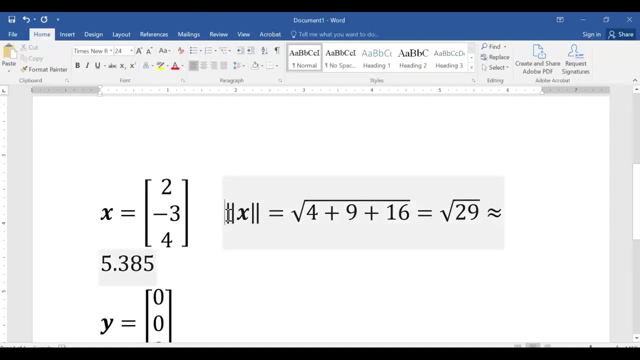 take the square root of 9 and call it 5.385, or you know roughly 5.385, then you could, But there's not a huge need to do that. Alright, Let's see if I can do this. 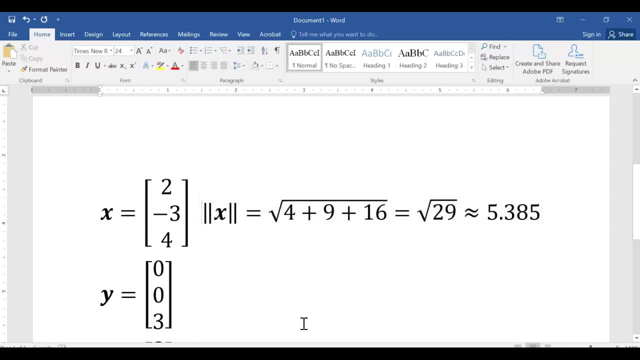 There we go. So there you go Now. length of y. let's take the length of y, So we take 0 times 0, plus 0 times 0, plus 3 times 2, so that is. 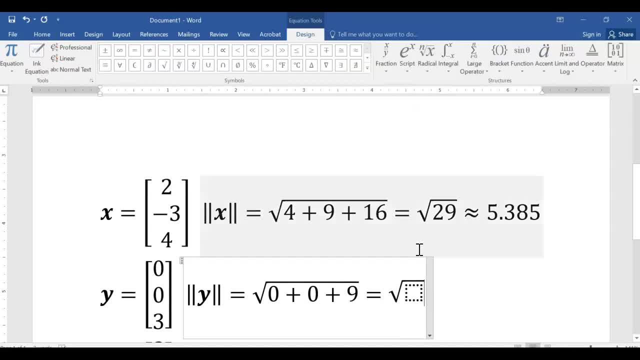 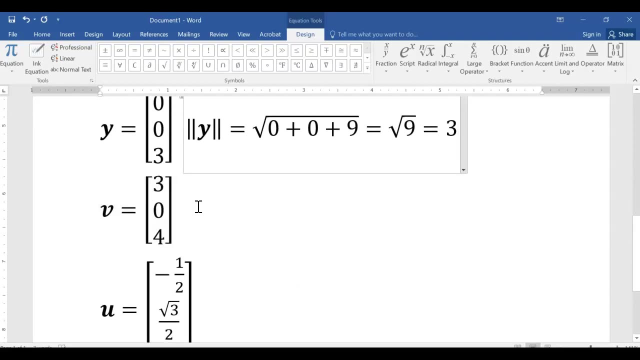 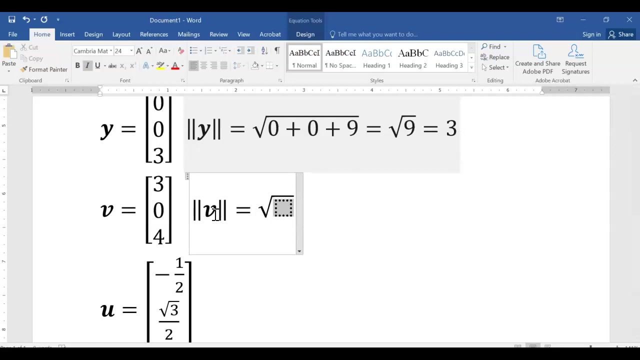 the square root of 9.. This one does simplify kind of nicely. The length of that vector is 3.. 3,, 0, 4 length of that vector which we called v is we take 9 plus 0,. 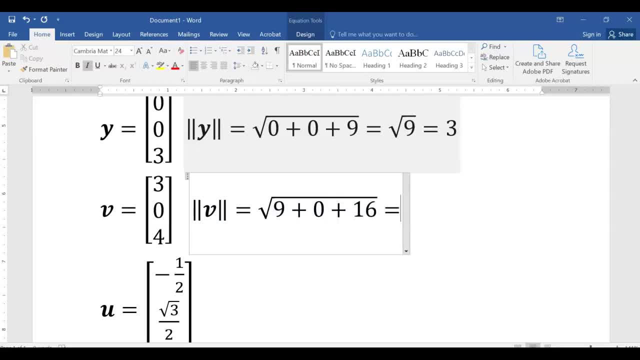 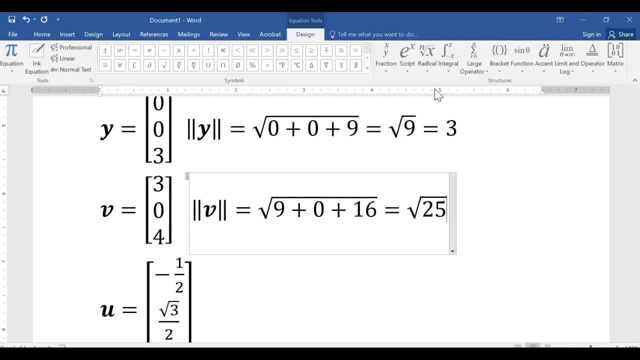 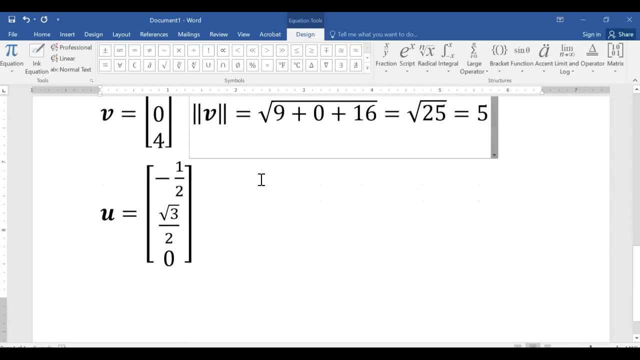 0 plus 16, which becomes the square root of 25.. So this one also has a nice length. It's length 5.. And then the length of u. so when I take negative 1 half times negative 1 half, 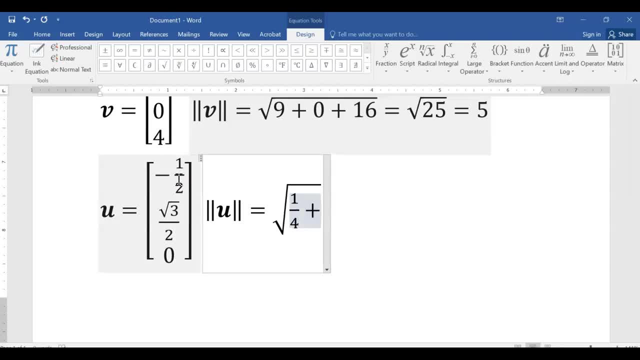 I get a positive 1 fourth. Plus when I take square root of 3 over 2, times the square root of 3 over 2, I get 3 fourths, And 0 times 0 is 0.. Now notice what we get here. 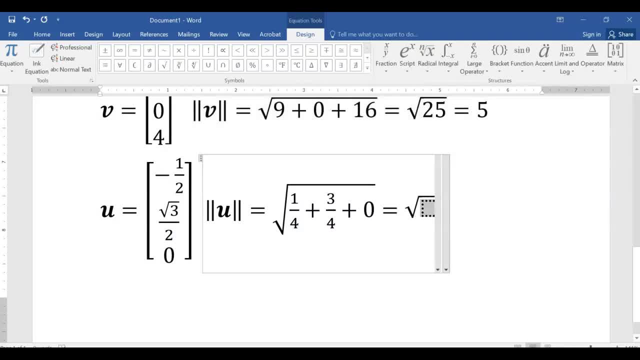 We get underneath the square root, we get a 1. And so that vector u is a 1. And so that vector u has length 1.. Okay, So that is the how to find length of a vector. 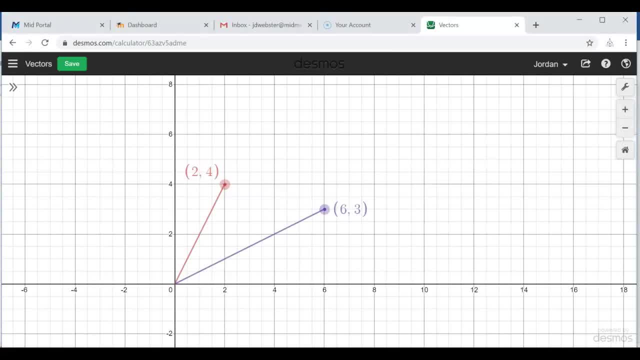 Now I want to just state that this is connected to the visual I had up earlier. The length of a vector is the length from the origin to the line, to the point. In this case it would be to the point 6, 3.. 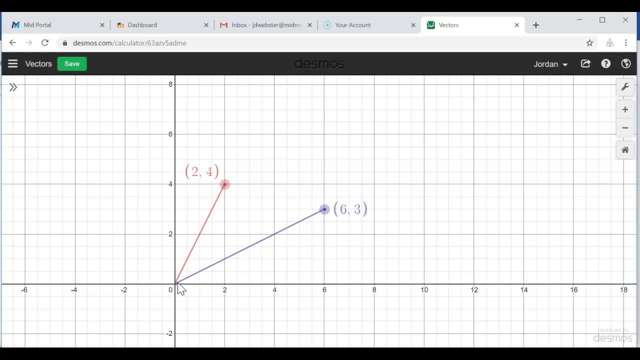 So if I'm talking about the length of vector 6,, 3, it is the length of that line from the origin all the way up to that point. So you do 6 squared plus 3 squared all under a square root. 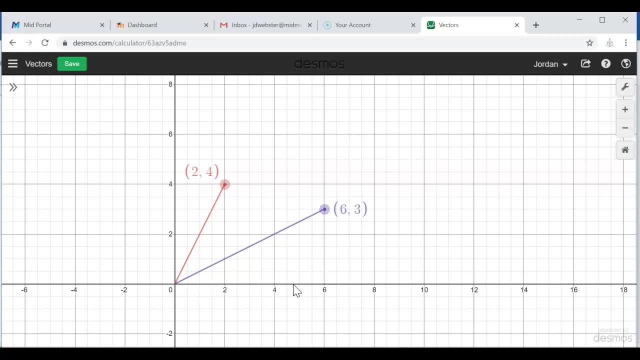 And, by the way, that should make sense because that's connected to the Pythagorean theorem. right This: 6, 3, if you think about what it's actually doing, There we go, It's create, we can create this right triangle. 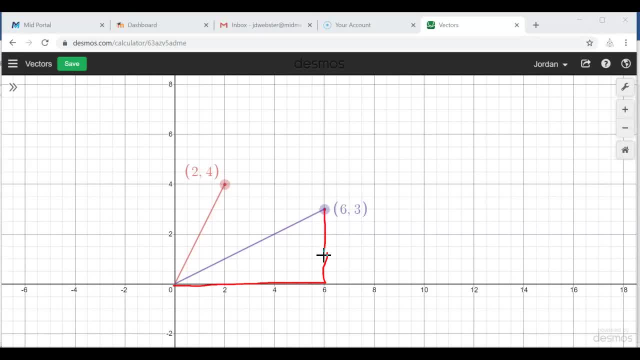 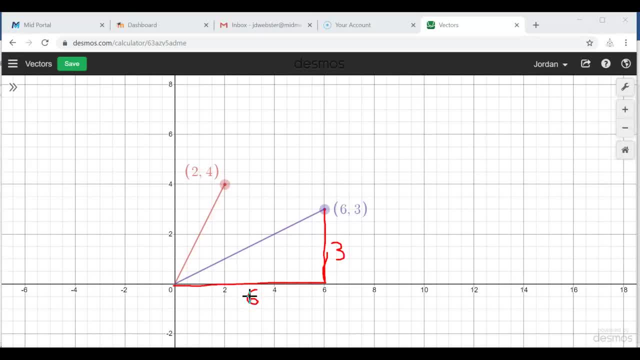 and this would be height length 3,, base length 6.. And we all know from the Pythagorean theorem that if you look at this right triangle the length of the hypotenuse is going to be c. if we call this length c, 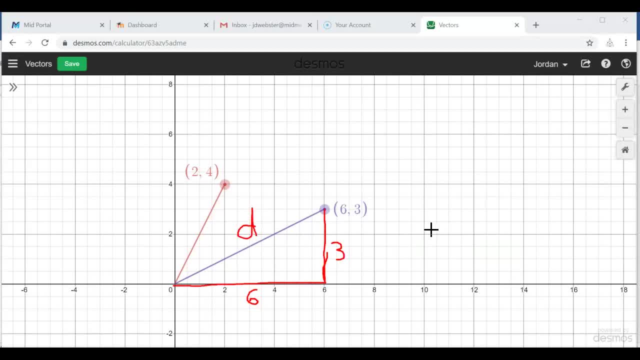 I'm going to call it d for distance. If we look at the distance distance squared- I'm drawing poorly, but that's okay- is going to be equal to 6, 3,. 6 squared plus 3 squared. 6 squared plus 3 squared. 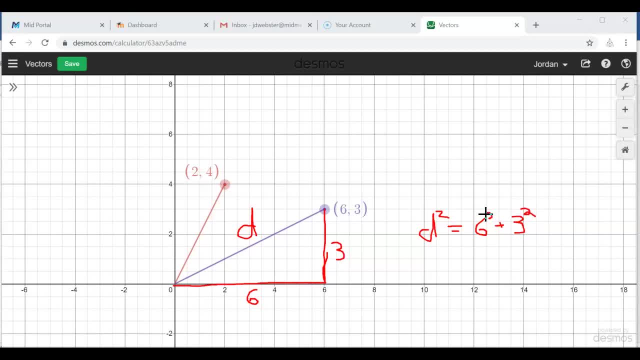 6 squared plus 3 squared. All right, That's just squared. It's ugly, But you see what's going on there, Okay, And so the distance is the square root. And so the distance is the square root of 6 times 6,. 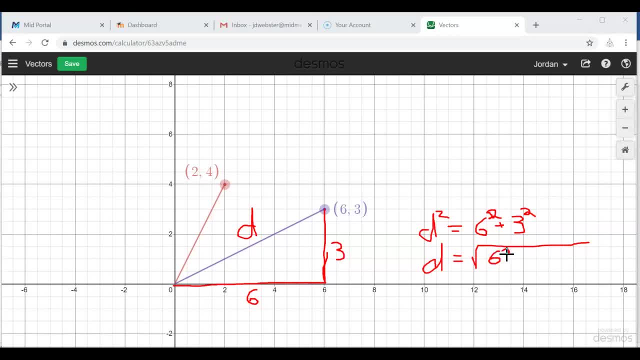 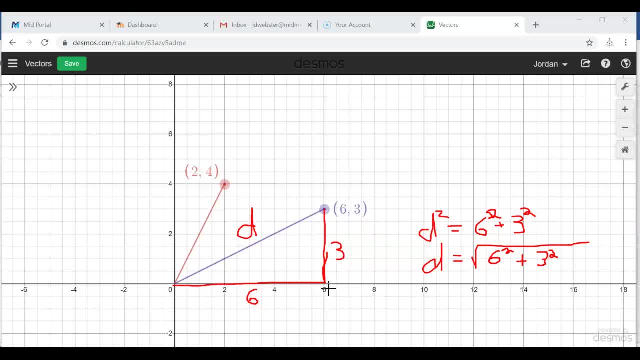 of the inner product of that vector. Okay, So this is the same distance formula that you know and you've seen before. that you know and you've seen before. I'm going to erase that because it looks awful, but But it is the same distance formula that we've dealt with before, or that you've probably dealt with before. 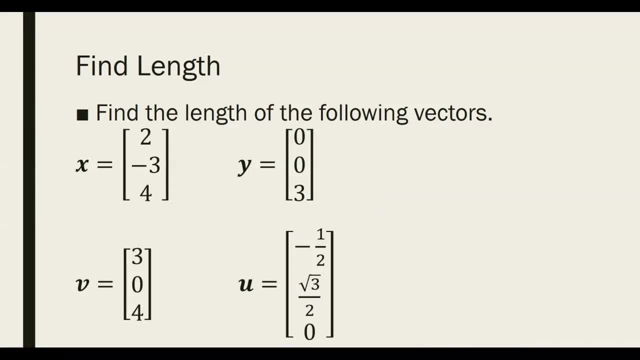 Alright, so we found the length of those four vectors. Now there are certain times in which it's nice to have unit vectors, okay, So any vector of length 1 is known as a unit vector. So in our previous slide we saw that the vector u had length 1.. 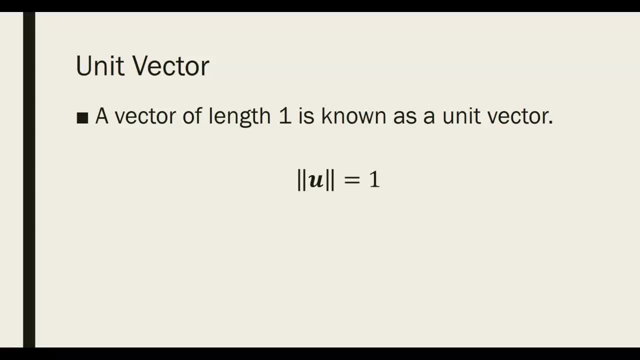 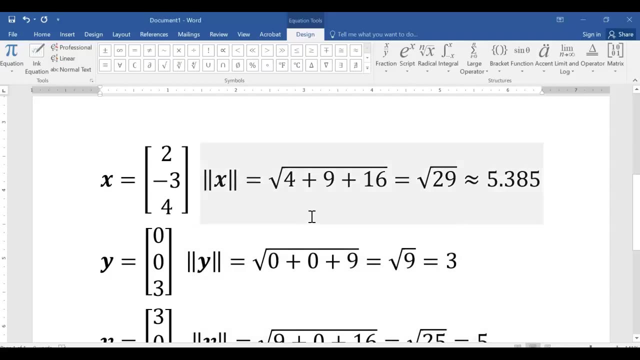 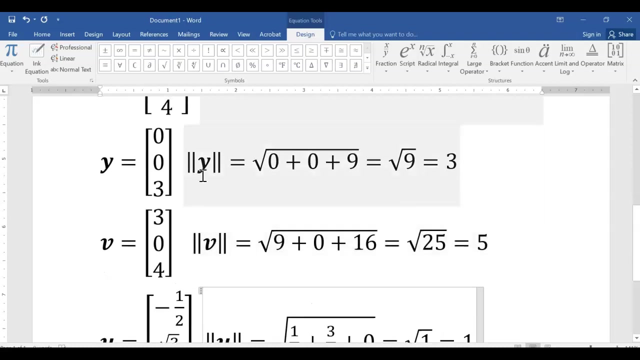 So the u from our previous slide would have been called a unit vector. okay, Now the other three vectors that we dealt with were not unit vectors. So obviously, x had length 5.385.. y had length 3.. v had length 5.. 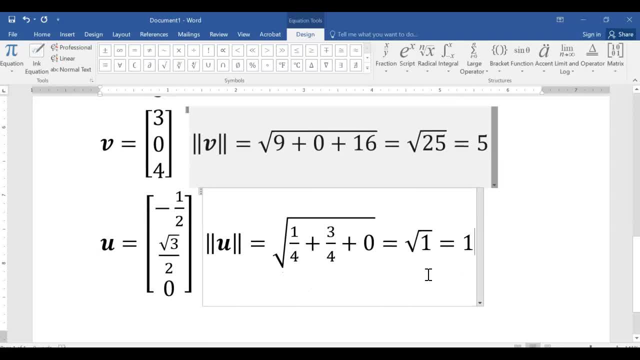 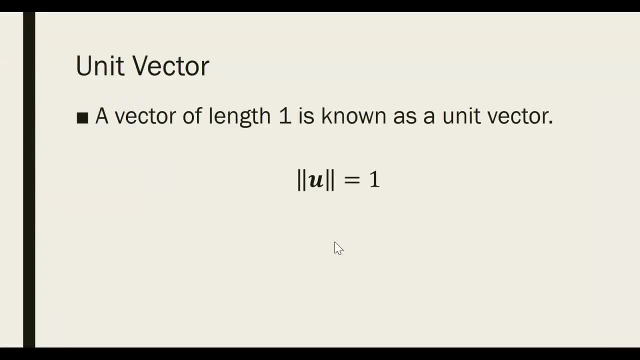 u was the only one that had length 1.. So what we can do is we can create unit vectors in the same direction as the vectors that we had before. So let's think about. Let's think about how we could create a unit vector in this same direction. 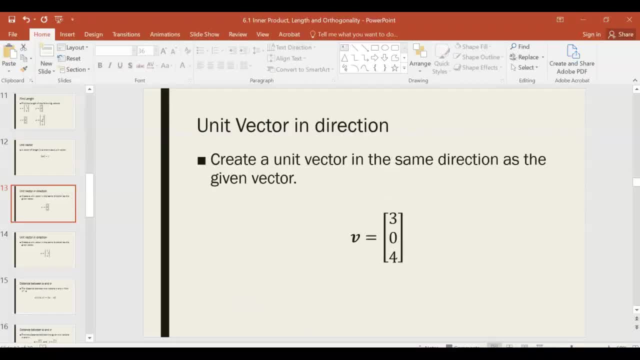 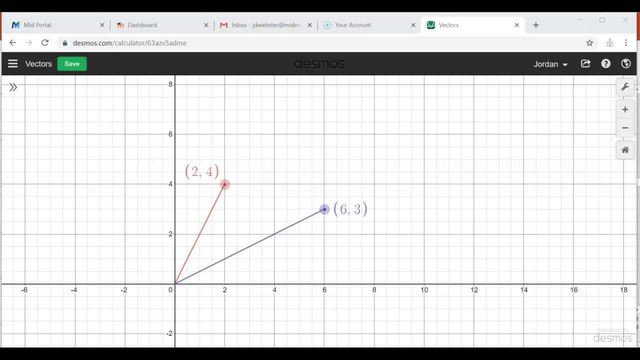 Now when I say in that same direction, let's go back to the 6-3 example. So when I say I want to create a unit vector in the same direction, basically I want a vector that goes out for a certain length. 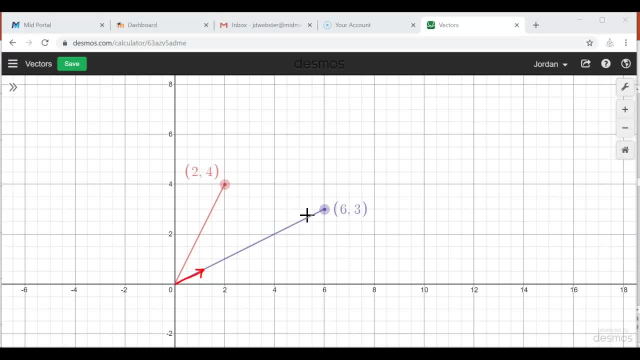 Along the path that 6-3 is taking, And then it stops when it hits length 1.. Now I drew this poorly because when it stops at length 1, who knows, It might be somewhere in here, something like that. 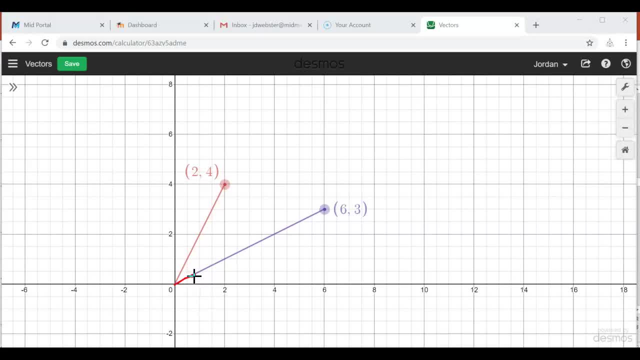 I don't know, Maybe closer to here, But it's not going to go all the way out to where x is 1.. The length of the vector needs to be Now, by the way, in this situation, my unit vector is just a scalar multiple of 6-3.. 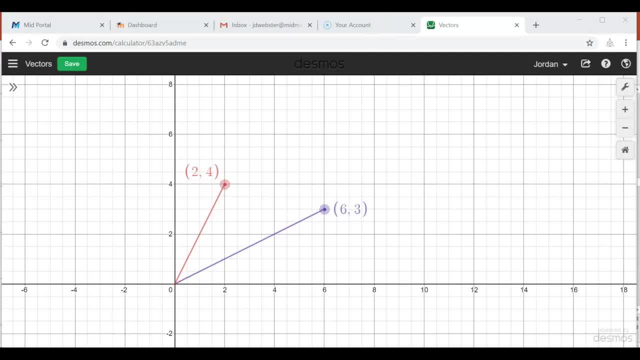 Obviously, if I started, So I'm going to make it just like that. Obviously, if I started my vector instead of using 6-3.. If I used a really short vector In order to get a unit vector, I'm going to have to scale it up instead of scale it down. 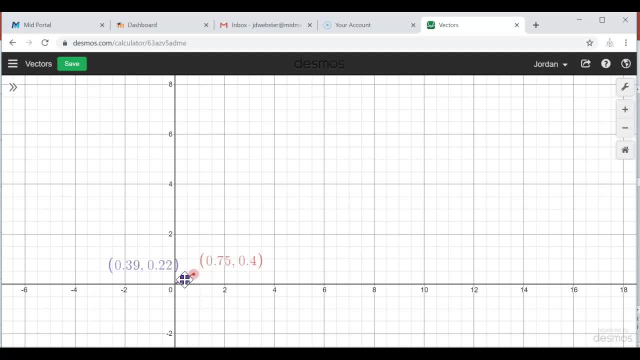 Does that make sense? But the point is it's in the same direction. So if I go to 6-3, roughly 6-3.. Unit vector is I'm going to scale that vector down to where my red vector has length 1.. 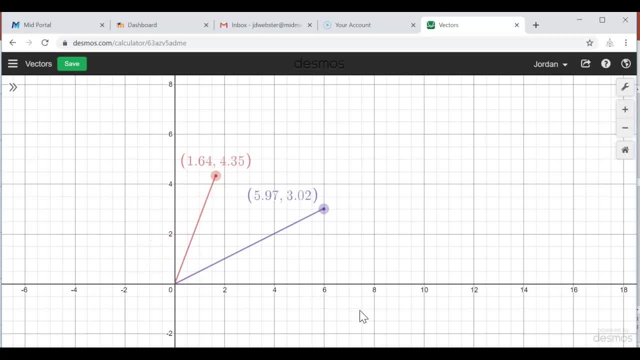 Alright, So, that's So, that's So. that's what's happening in the sense. So when I say scale it down or in the same direction, in the same direction means it's along the same path, In other words, it's going to be a scalar multiple. 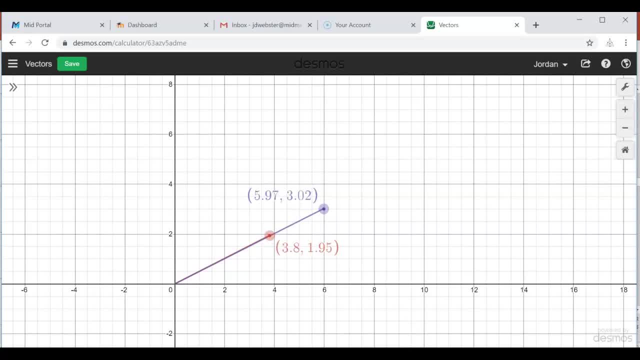 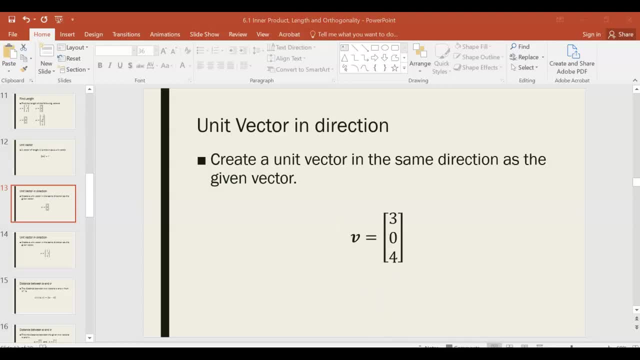 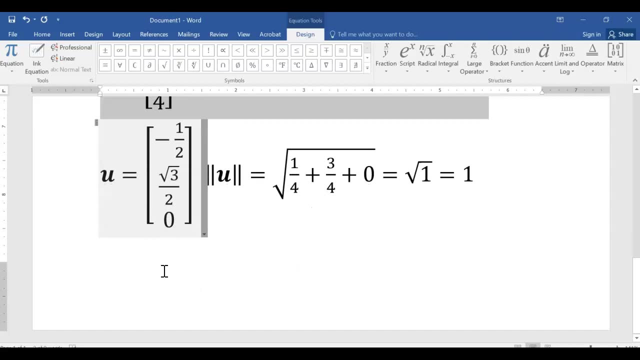 These two are going to be scalar multiples of each other, So let's create one in the direction of 3-0-4.. So we've taken our v, which we know has length 5.. Let me get to a new page there. 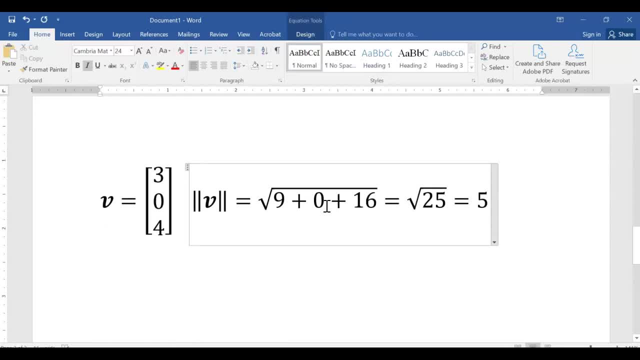 So we've taken our vector, which we know has length 5.. Now, if we want to make sure this has length 1, all we have to do is multiply v by some scalar. Now, what scalar do we need to multiply it by? 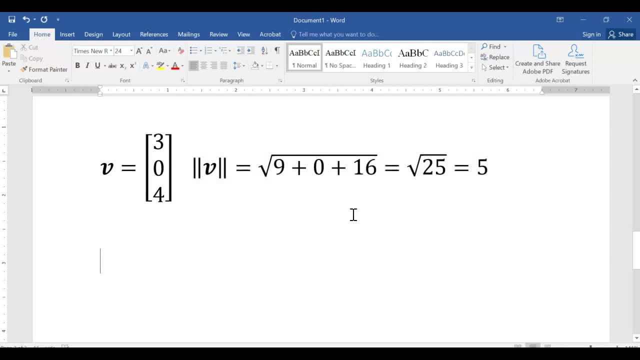 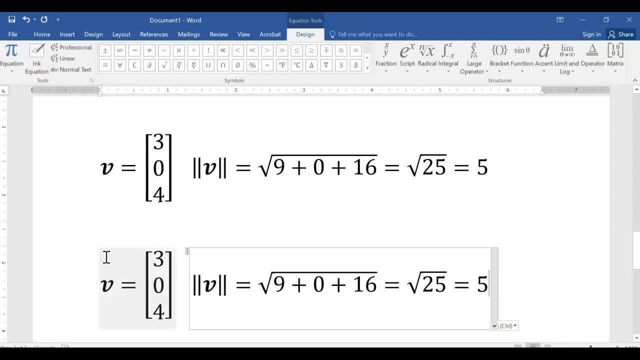 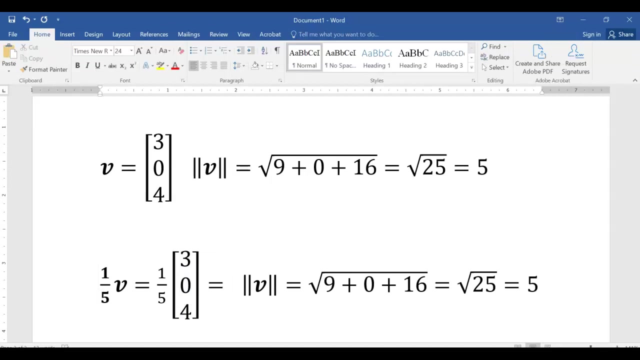 Well, we need to multiply it by 1-5.. Think of what that's going to do. So let's take 1-5 times v, Okay, So what we get as a vector is 3-5,, 0,, 4-5.. 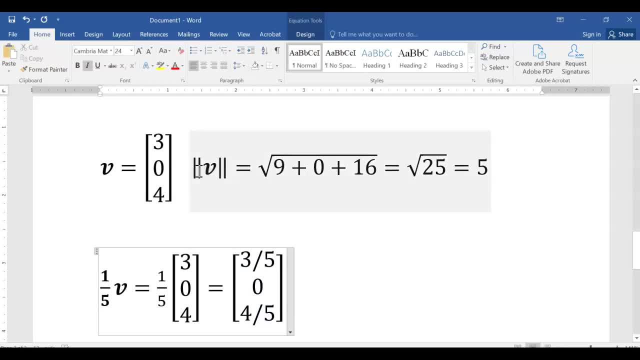 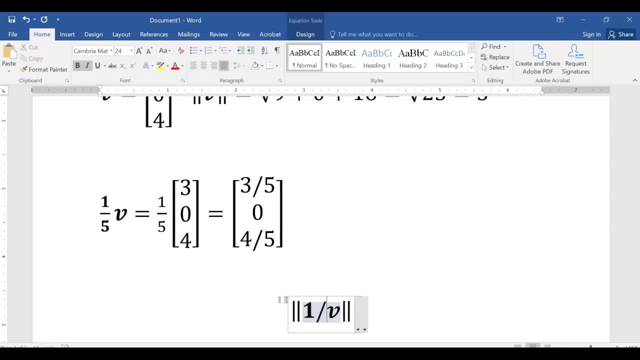 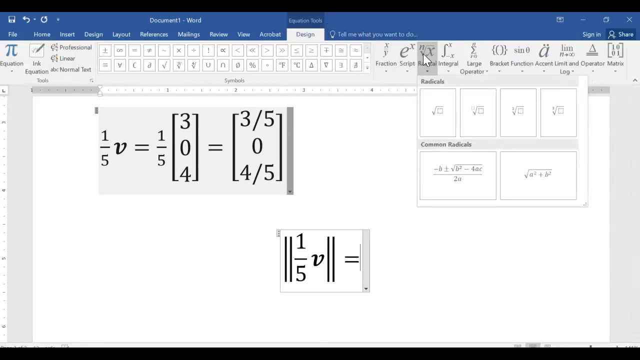 Now, if I think about the length of that vector, the length of 1-5 times v. Do it down here. There's some things that are bold, that don't need to be, but that's all right. So length of 1-5 times v is going to be equal to the square root. 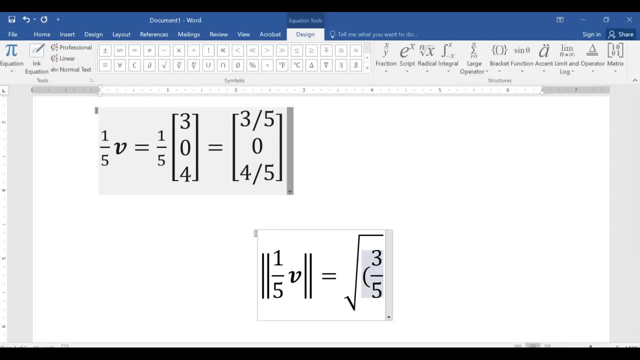 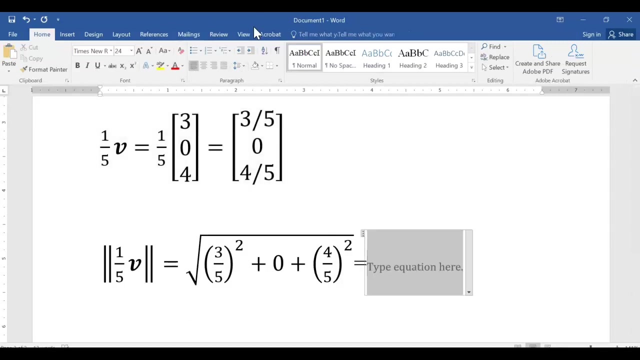 If I take 3-5 and square it- Oh, that's ugly, Okay, That's better. And then plus 0 squared, plus 4-5 squared, What you'll notice is that we end up with the square root: 3 squared is 9.. 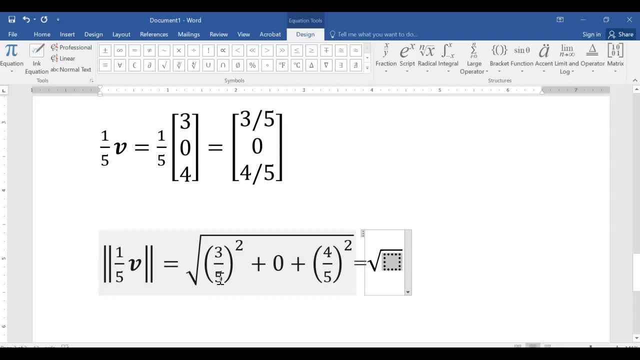 4 squared is 9.. 4 squared is 16.. 5 squared is going to be 25.. So we're going to get 9 over 25 plus 0 plus 16 over 25, which 9 plus 16, is just 25.. 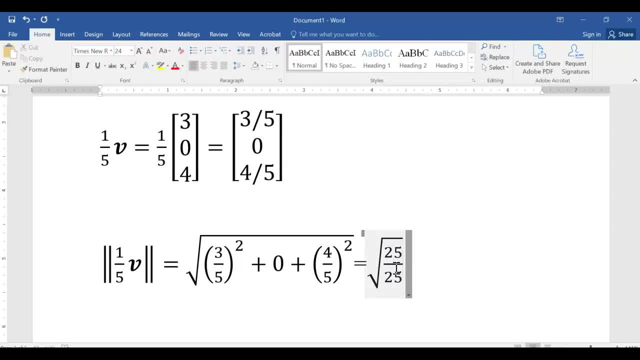 So I end up with 25 over 25, which is obviously 1.. And when I take the square root of that, I still get a 1.. Okay, Okay, Nope, That's better. Okay, So there you go. 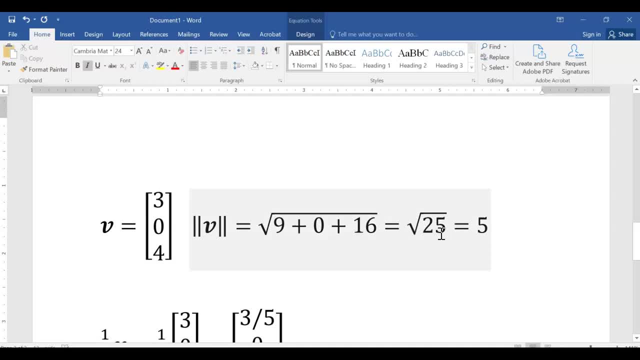 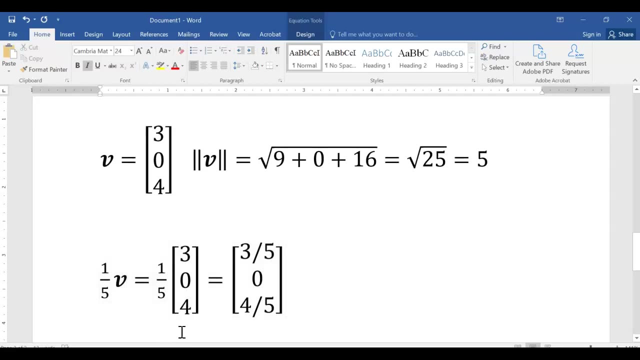 So basically, all I do when I want to find a unit vector is I take the length, take the reciprocal of the length and multiply it times the vector itself. That will be a unit vector in the same direction as v. So what I'd like you to do is try another one. 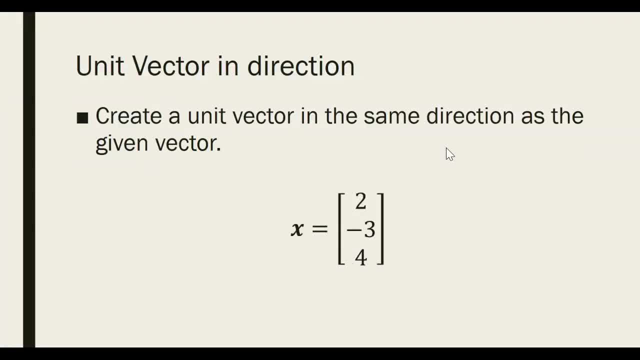 I want you to go ahead, create the unit vector in the same direction as the x- This is the same x we dealt with a couple of slides ago- And then, once you've created that unit vector, see that it indeed works out. In other words, see that when you plug in 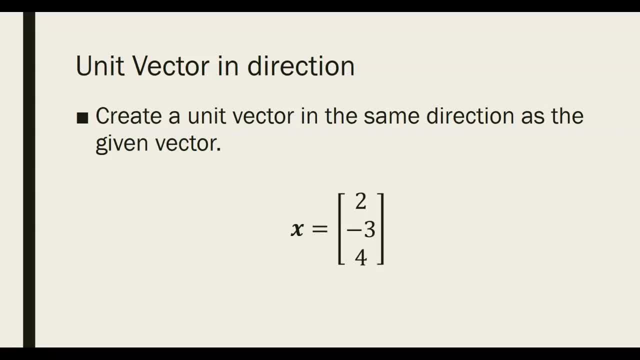 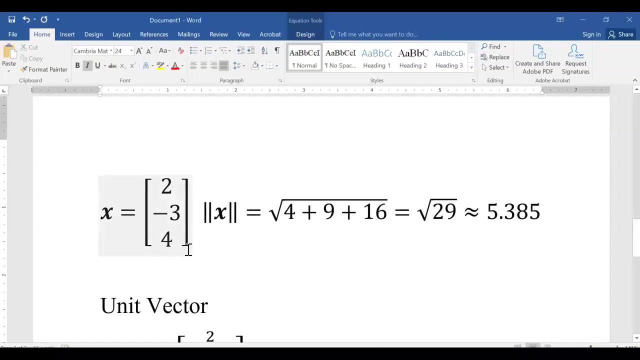 or when you calculate the length of whatever unit vector, we found that it comes out as length 1.. All right, So hopefully you went ahead and did that Now. from the previous work we saw that the length of x is square root of 29.. 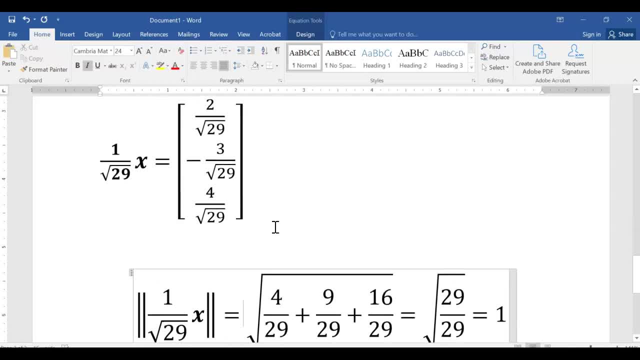 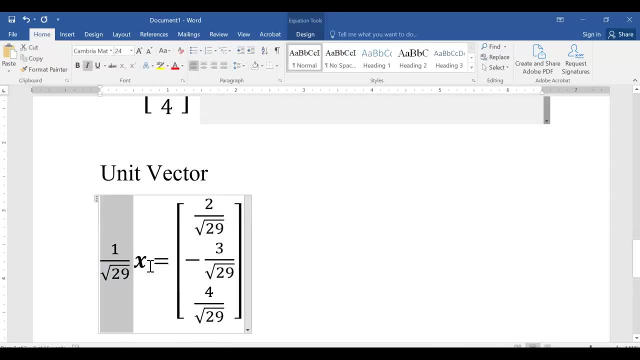 So all we would have to do to create a unit vector, it should be to take 1 over the square root of 29, and then multiply that times x. Now, if you do that, basically all these entries are just going to be divided by the square root of 29.. 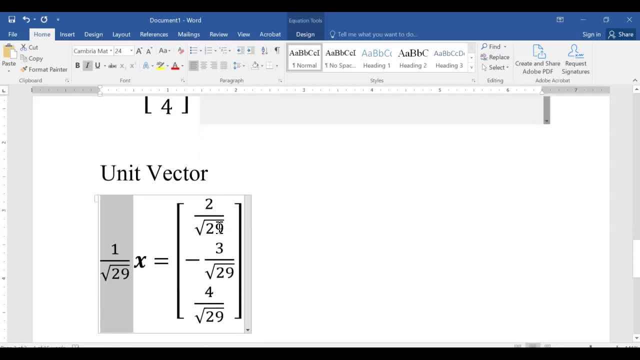 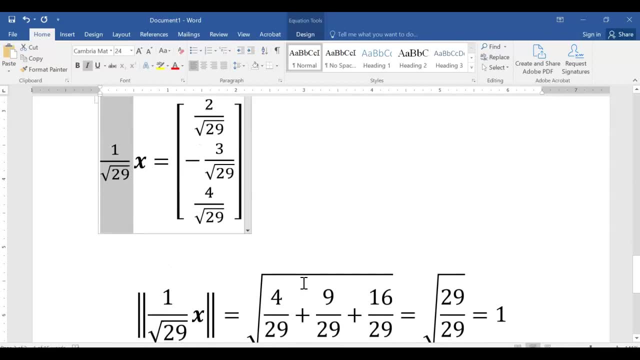 So we're going to get entries which are 2 divided by square root of 29,, negative 3 divided by square root of 29, and 4 divided by square root of 29.. All right, So that is the unit vector that is in the same length. 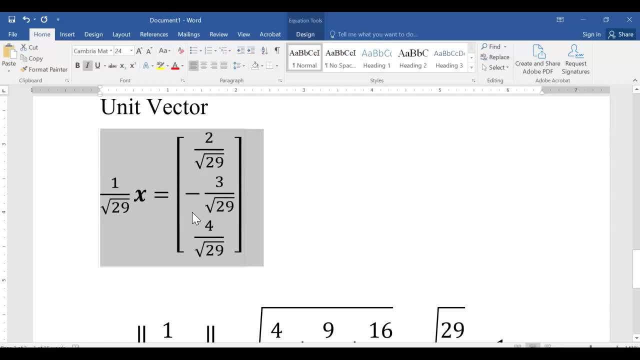 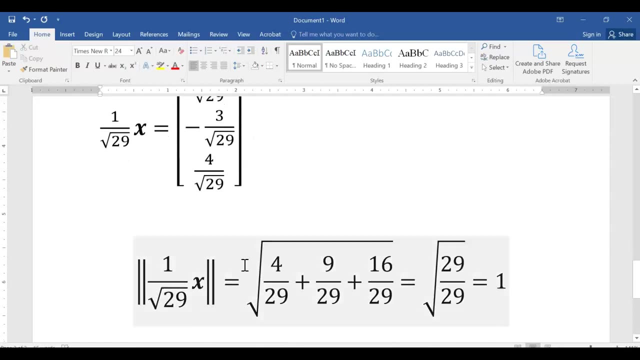 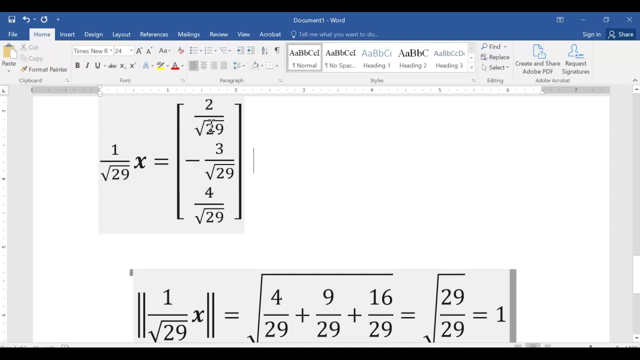 excuse me, is in length 1,. hopefully It'll have length 1, and it will be in the same direction as x. Now you can confirm that this has length 1 by just taking the length. so in our product, 2 over root, 29 times another 2 over root, 29. 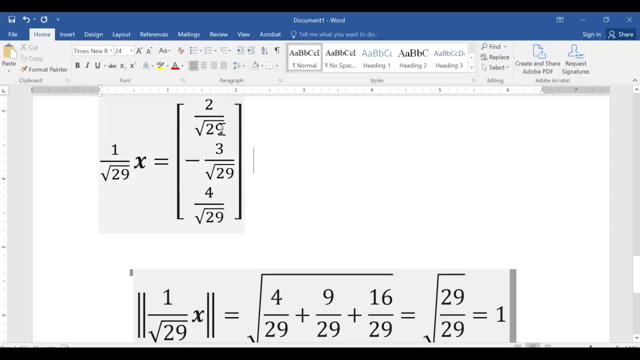 is going to give me a 2 times 2 is 4, square root of 29 times square root of 29 is just 29.. So you're going to get 4 over 29.. When you take your first entries, multiply them together. 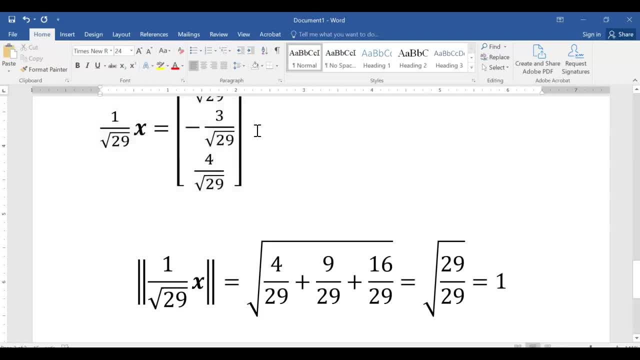 negative 3 over root 29 times another negative 3 over root 29 is going to give me: 3 times 3 is 9, divided by 29.. 4 times 4 is 16, divided by 29.. So what you'll see is you get 4 over 29,, 9 over 29,, 16 over 29.. 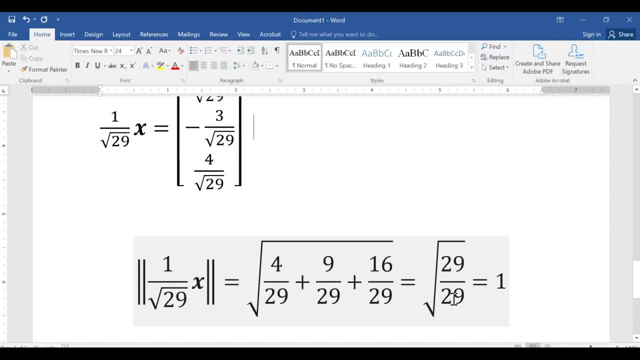 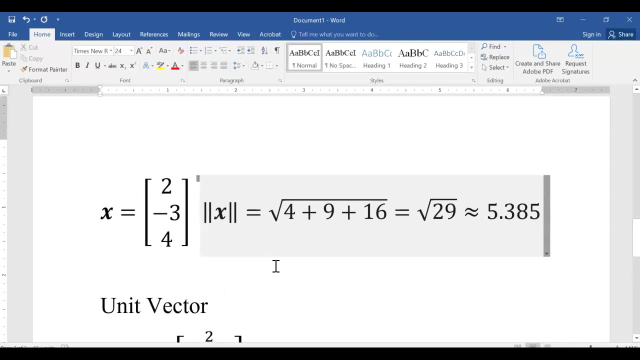 4 plus 9 plus 16 is 29 over 29.. And obviously that reduces to just 1.. So what I'm saying is that if you ever wanted to have a test sort of, scale down your vector and make it, instead of length, 5.385. blah, blah, blah. 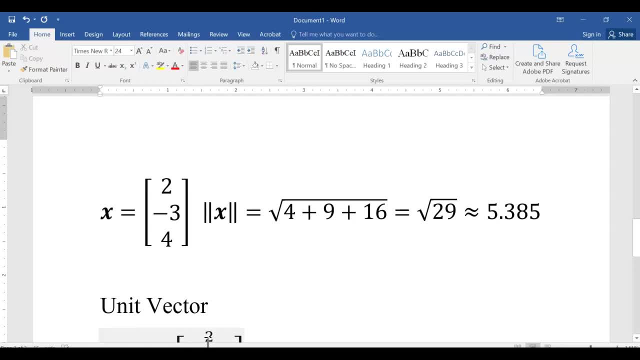 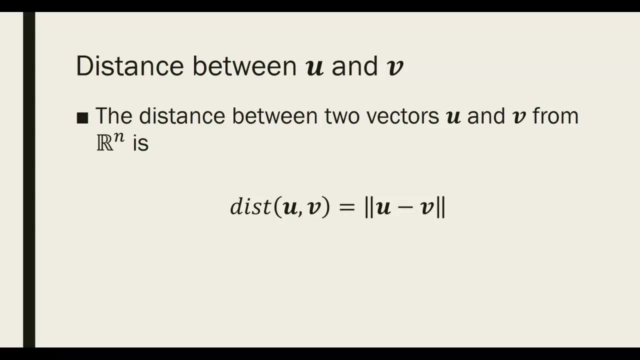 then all I have to do is multiply it times the appropriate coefficient. All right, so for any non-zero vector I can do that. Now, another concept that we look at in Section 16, Section 161, is the concept of distance between two vectors. 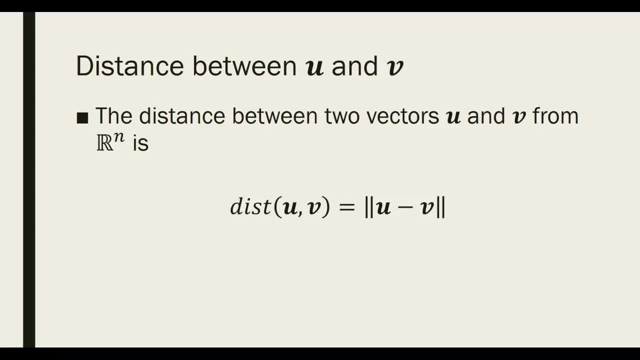 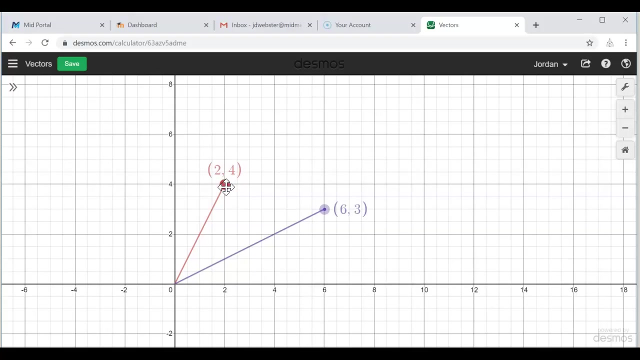 So the distance between two vectors is basically the length of the vector we would create when we subtract the two vectors. Now we can take a look at what this is actually doing here. So let's go back to my drawing. Let's go back to my drawing where I had the vectors 2, 4, and 6, 3.. 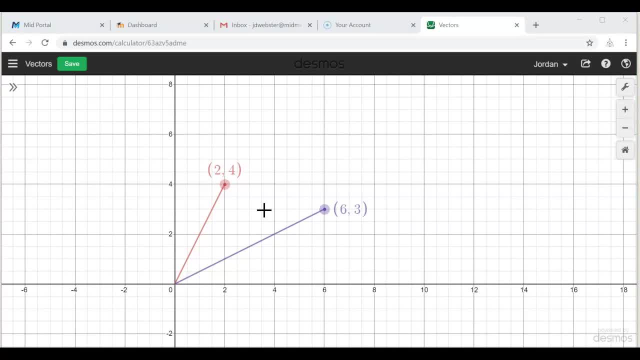 Now, what would the distance between those two vectors be? Well, I'll simply put: the distance between 2, 4, and 6,. 3 is the distance of, if I were to draw them straight, the straight line between these two. 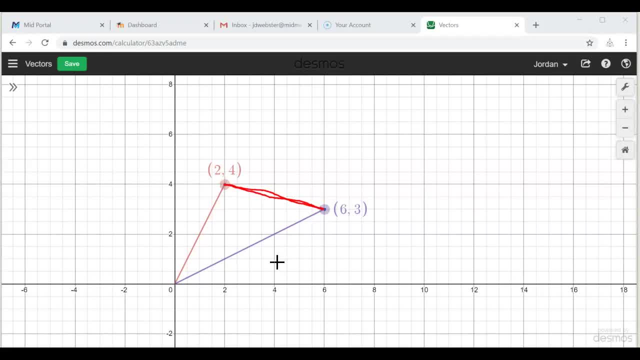 In fact, you can see that if you subtract you would get those, Depending on the way you subtract. So the distance between those is the distance between the point that they end at, the point that this one ends at and the point that this one ends at. 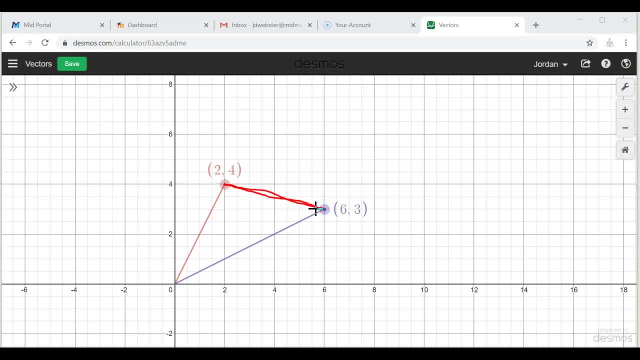 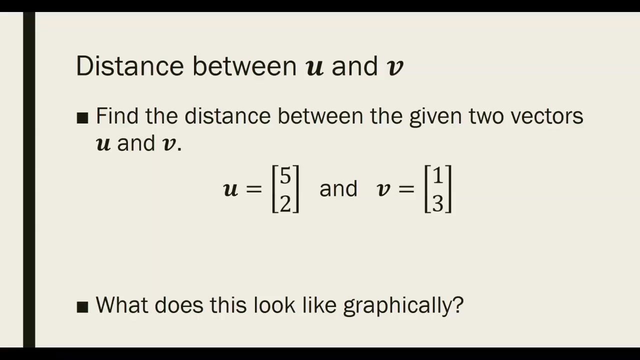 All right, so that's the distance of that line is, in fact, the distance between the two vectors. Okay, So let's go ahead and calculate all that. Why is this not? I want you to find the distance between those two vectors. 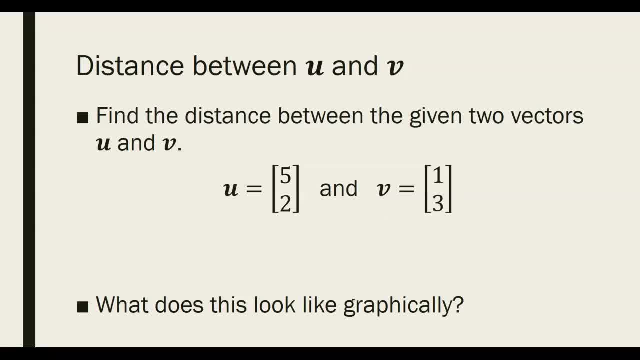 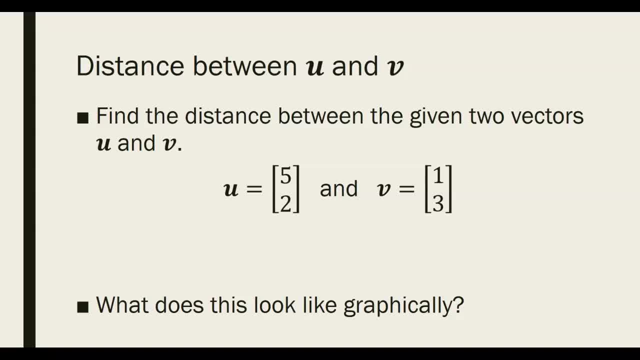 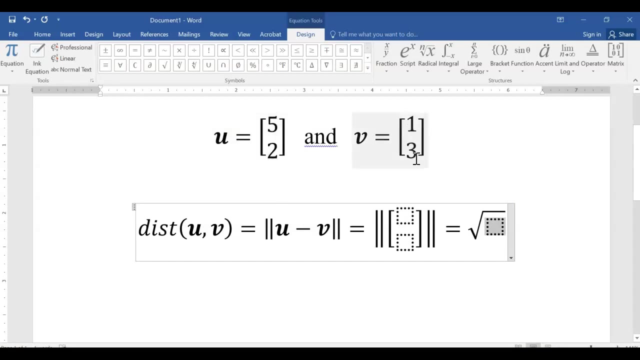 and then think about what that looks like graphically, Push pause on the video and go ahead and do that. All right, so hopefully you went ahead and did that. So here's what we did. We got 5,, 2 and 1, 3.. 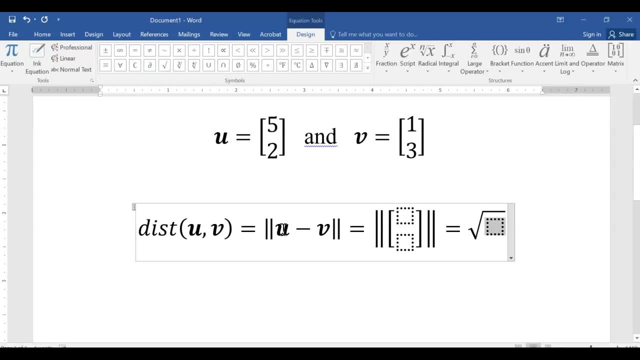 we're looking at the distance between those two vectors. So we take and subtract: 5 minus 1 is 4.. 2 minus 3 is negative 1.. By the way, you'll notice that the distance from uv to vu is exactly the same. 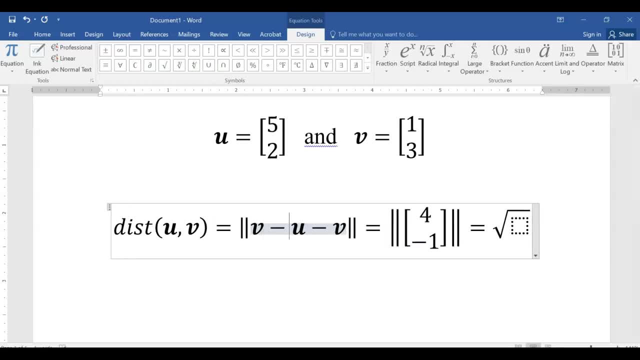 because if I would have subtracted v minus u, all it would do is change that positive 4 to a negative 4 and that negative 1 to a positive 1.. But when we take the length, since we're squaring each entry- 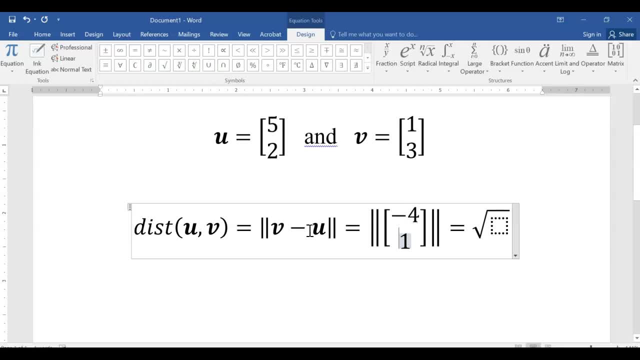 taking each entry times itself. that really doesn't change anything. So u minus v, I'll do it that way. That turns into a positive 4 and a minus 1.. So that's the difference. So that's the difference. Now, length of 4. negative 1 is going to be the square root. 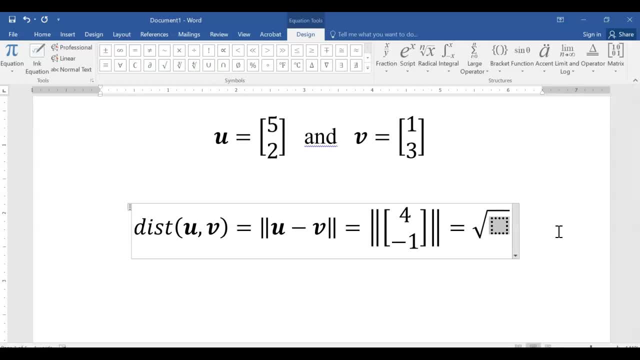 of the inner product of 4, negative 1 times itself. 4 times 4 is 16.. Negative 1 times negative, 1 is 1.. So what we end up with is that the length or the distance between u and v is the square root of 17.. 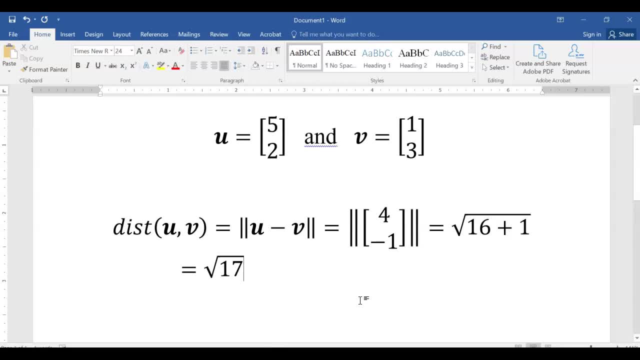 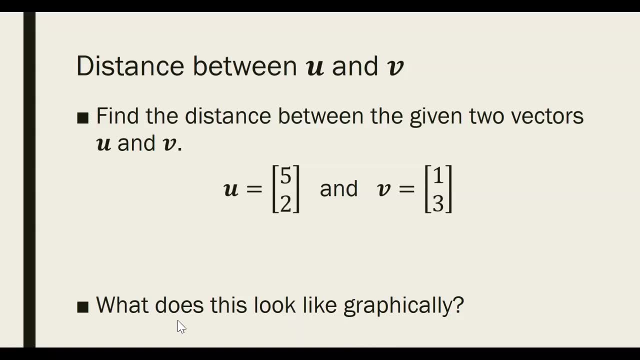 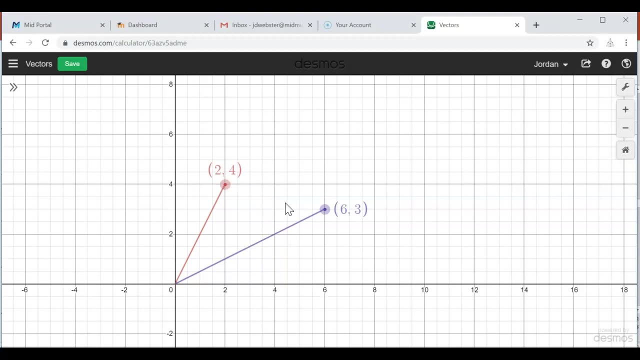 Alright, So that's how it goes. Now, what's this look like graphically? We kind of already went over what it looks like graphically, But basically it's the length of that section again, from tip to tip. I'm not going to draw that, but tip of the vector to tip of the vector. 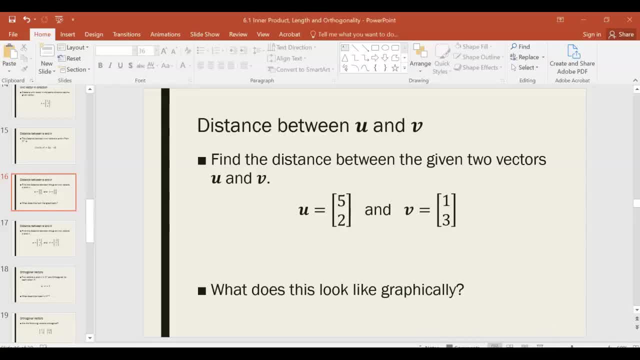 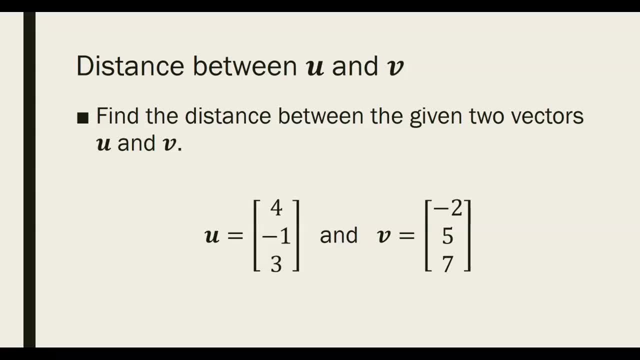 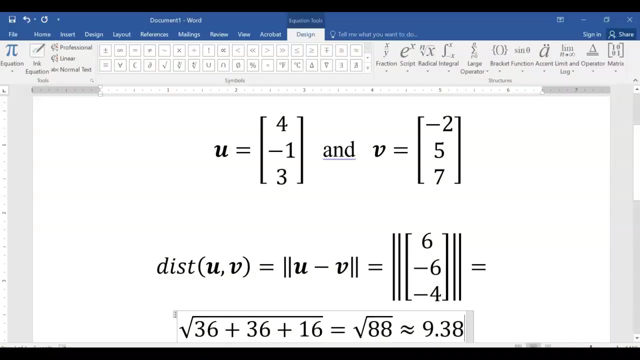 So there we go. I want you to calculate the distance between these two vectors. So push pause on the video, calculate the distance between these two vectors and R3, and then I will do it as well. Alright, Alright. so here it is. 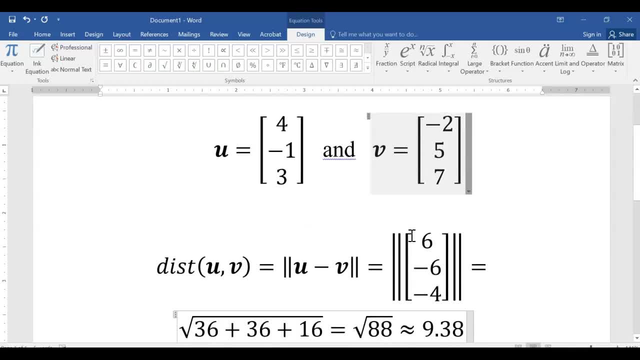 So we take u and v and we're going to subtract them. Now, be careful when you subtract, because we have negatives around here. So I do 4 minus negative 2.. Subtracting a negative is like adding 2.. So I end up with a 6.. 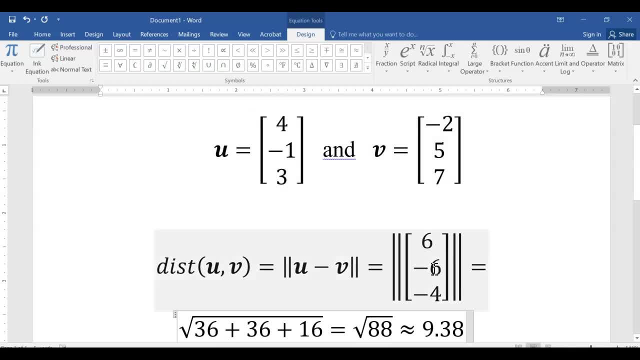 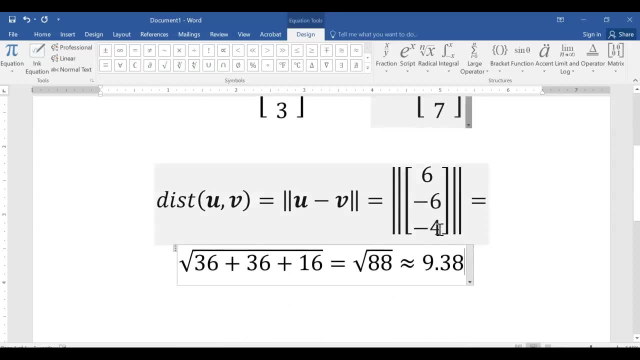 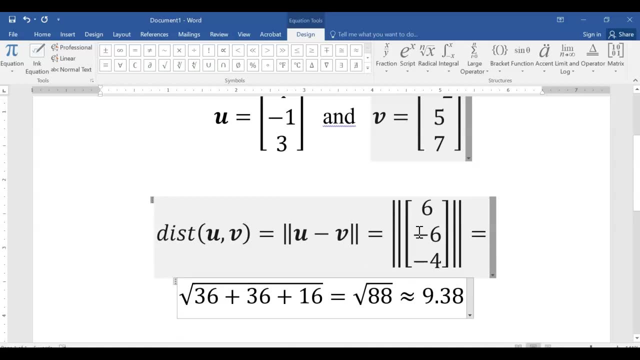 Negative: 1 minus 5, I end up with a negative 6. And 3 minus 7, we end up with a negative, Negative 4.. By the way, if you just subtracted v minus u, you would have ended up with just changing the signs on each of these entries. 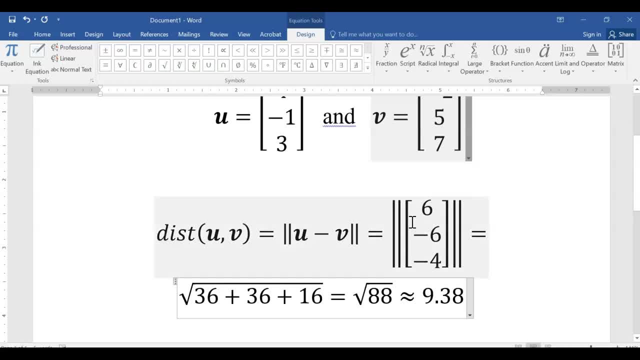 So what we do find the length, Take 6 times itself, which is 6 times 6, is 36.. Negative 6 times a negative. 36 is a 36.. Negative 4 times negative. 4. Is a 16.. 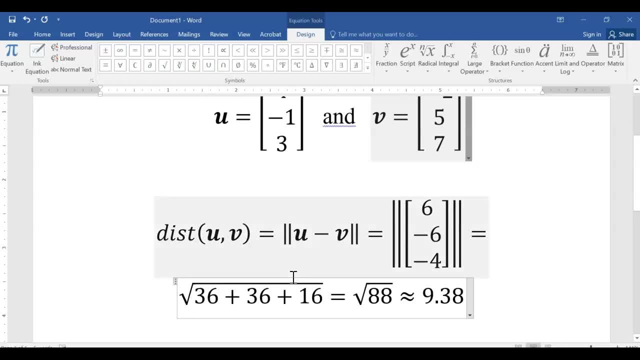 We take the square root of all of that and we see that the distance between this u and this v is the square root of 88.. Now, the square root of 88 is an irrational number. So if you wanted to simplify that and write something like 2 root 22,, that's fine. 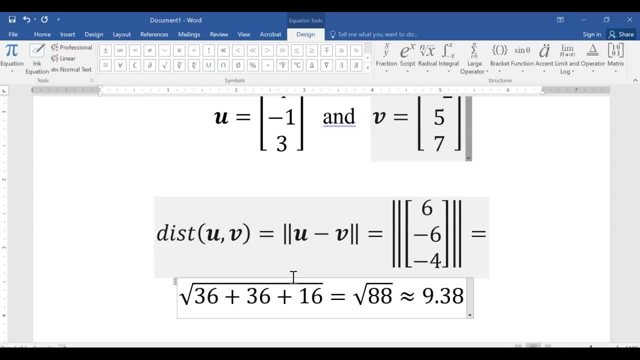 But square root of 88 is perfectly acceptable. Um, to have a length If you wanted to round it. um, if you rounded it to 2 decimal places, 9.38 would be rounded to 2 decimal places. Alright, so that's the idea of distance. 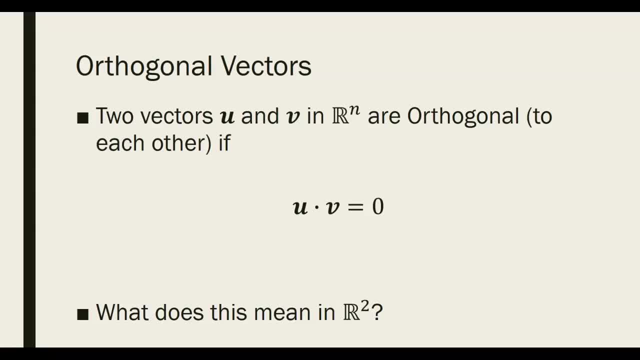 Now we get into what's going to be the major focus of chapter 6. And that is the concept of orthogonal Vectors. So we say that two vectors are orthogonal if the inner product is zero. So if the inner product is zero, then those two vectors are orthogonal. 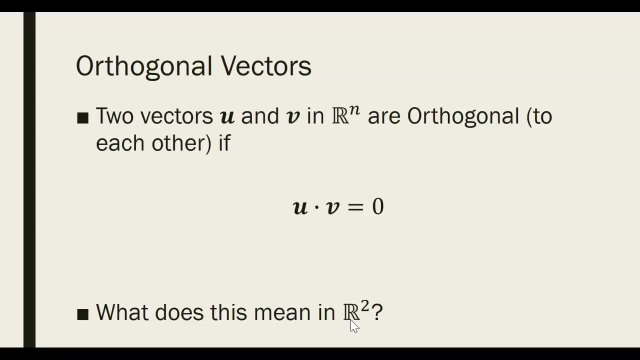 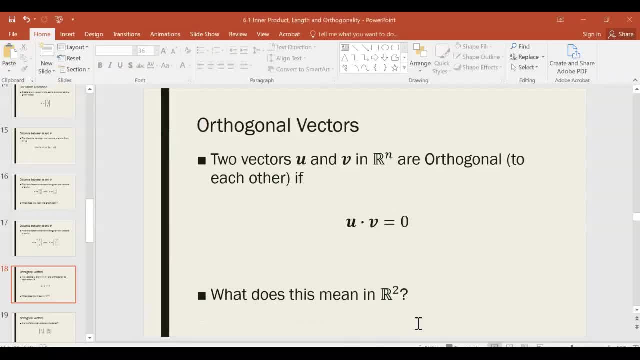 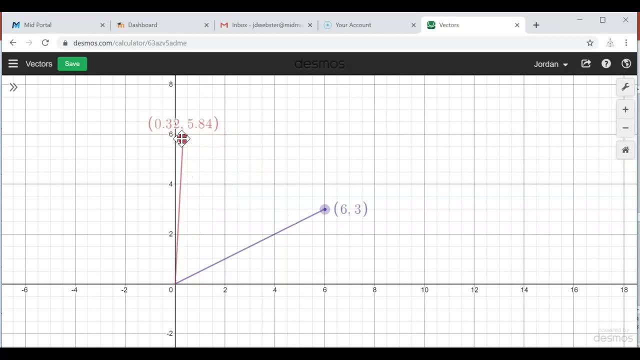 Well, let's take a couple of. Let's take a look at R2.. So orthogonal vectors in R2 are ones that hit at a 90 degree angle. So, if I've drawn this right, if they hit at about a 90 degree angle in R2,. 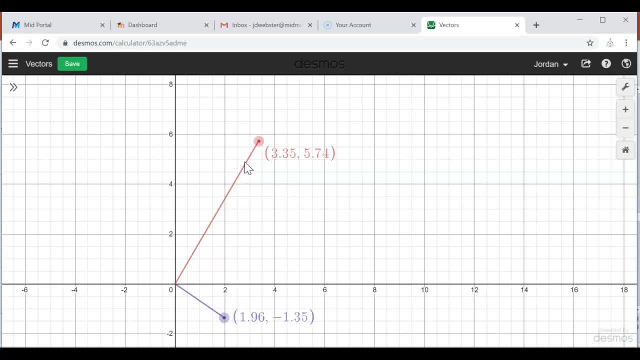 then they are orthogonal. If they don't hit it on a 90 degree angle, then they're not orthogonal. So, for instance, these two vectors are not orthogonal. However, this one and this one- something like that- appear to be orthogonal because they appear to hit at 90 degree angles. 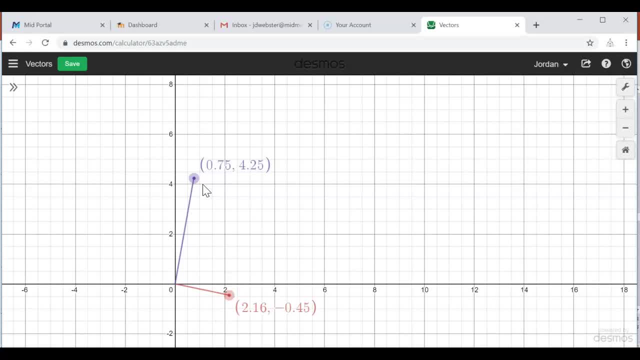 So there you go Now. in general, there's the- oh, how do I say? In general, there's something about this that you can, you can extend to R3 and R4 and R5, and it has to do with the length. 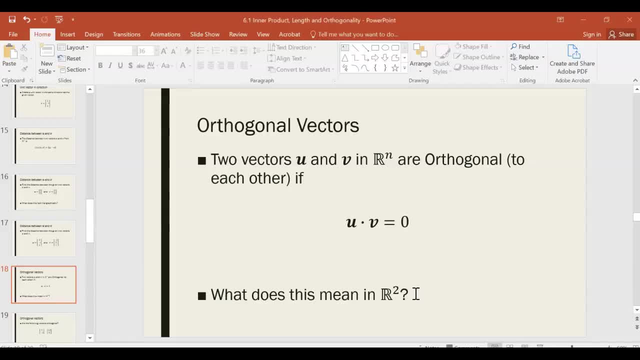 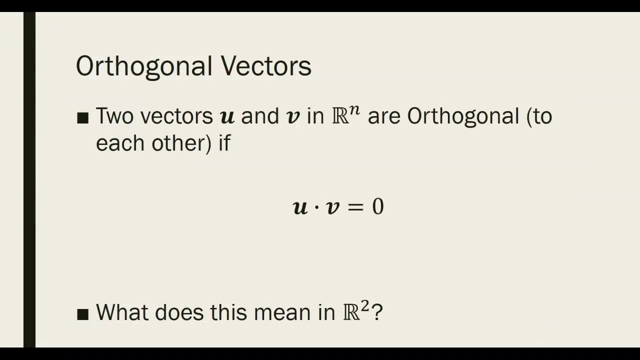 But basically, what we need to understand is that orthogonal vectors are somehow akin to perpendicular vectors in R2.. And we can see when they're orthogonal, because when they're orthogonal, the inner product is zero. So I want you to go ahead and see if these two vectors 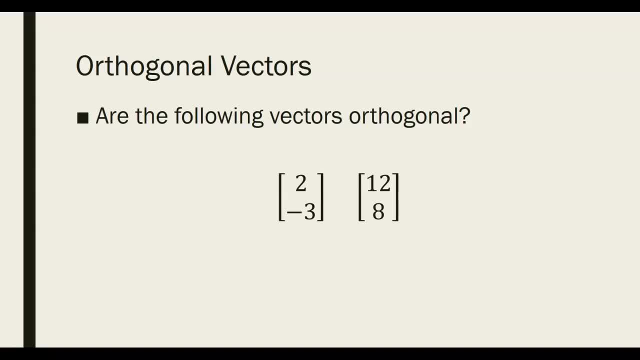 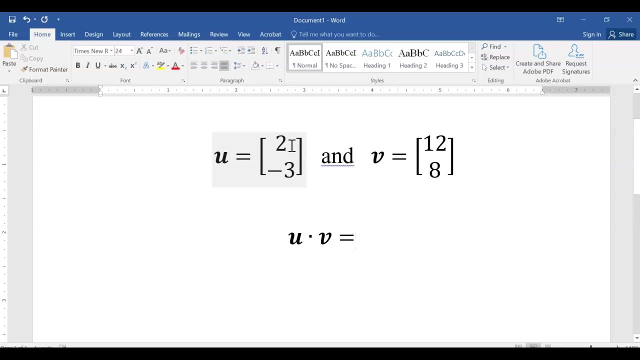 are orthogonal, Alright, so hopefully you did that Alright. so we take these two vectors and we do this, And in product I'm calling them u and v, just to make it a little bit shorter. You can call them whatever you want. 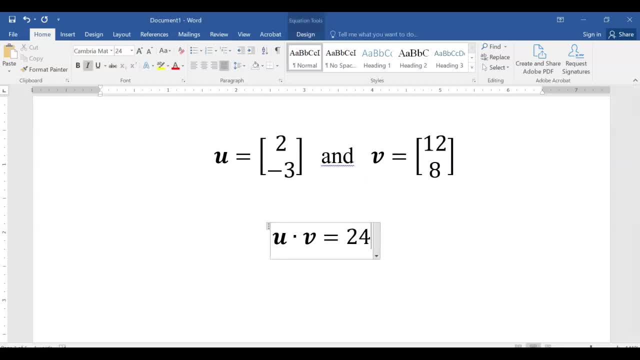 2 times 12 is equal to 24 minus 3 times 8. also, well, that's actually equal to negative 24.. So when you add them up, you get a zero. So these two vectors are in fact orthogonal. And if you graphed those two vectors, 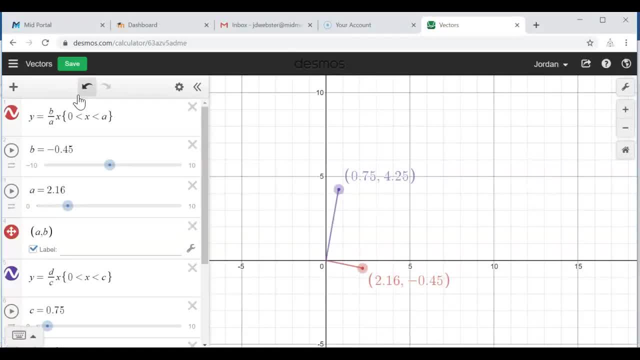 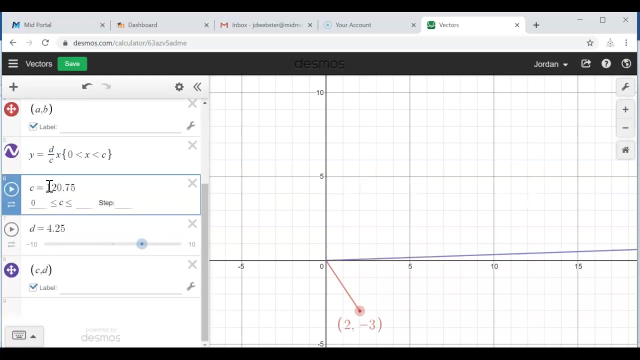 let's try to graph those. This is going to look a little bit ugly, But that's okay. We say 2, and then negative 3, and we'll go to 12, 8, and so what we see is that. let me scroll back a little bit. 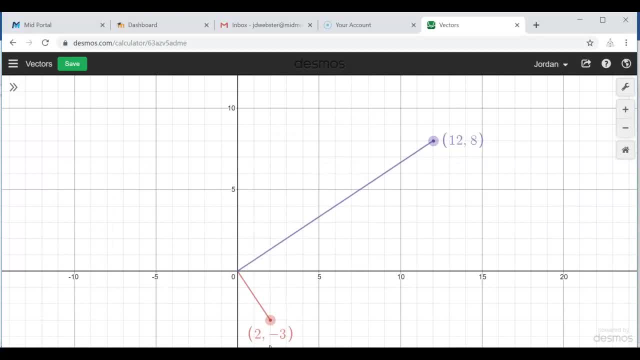 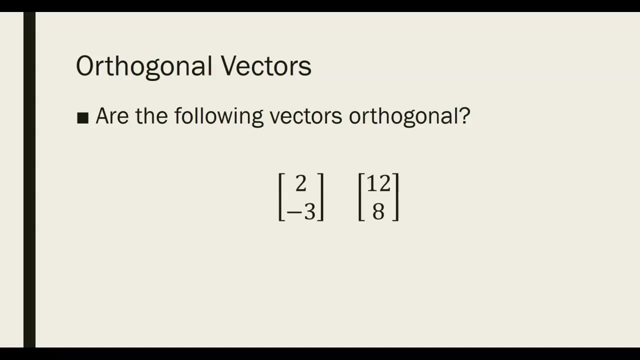 12,, 8, and 2, 3 are in fact orthogonal, so they are perpendicular. At least they look perpendicular. Okay, Alright, now again, that concept of orthogonality extends to other dimensions and we're going to look at that. 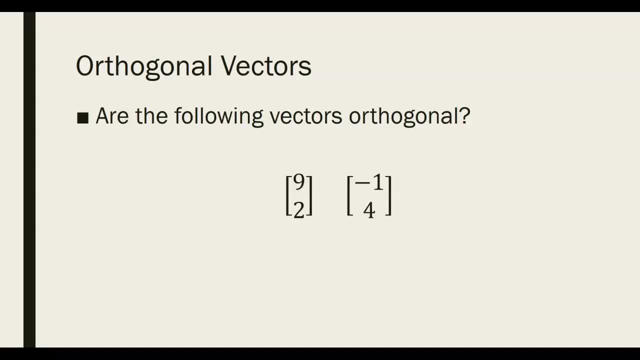 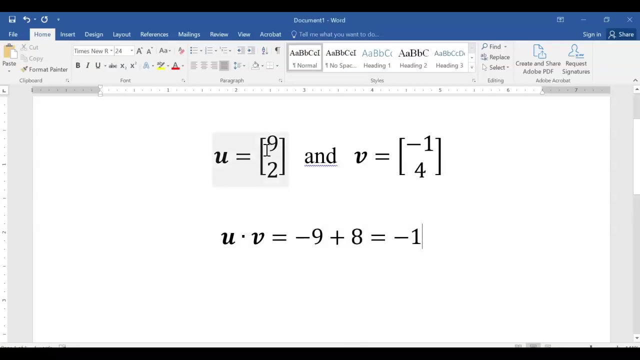 in a little bit later, And so on and so forth. I want you to test if these two vectors are orthogonal: 9, 2, and negative 1, 4.. Alright, so 9, 2,, negative 1, 4. 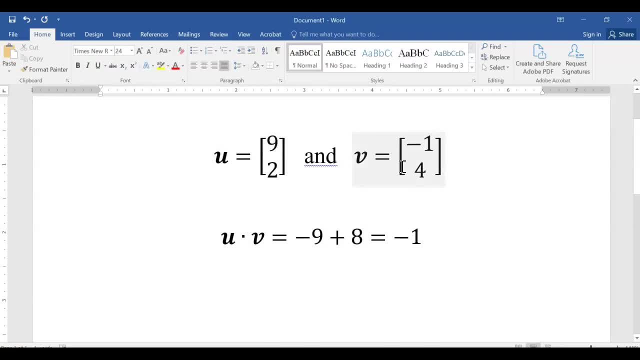 when I multiply 9 times negative 1, I get negative 9.. 2 times negative: 1,, 4. I get 8. You end up with a negative 1. So obviously these two vectors are not orthogonal. By the way, 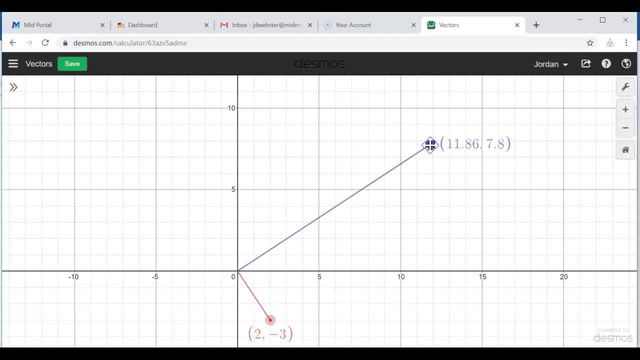 if we looked at- I'll try to do this- the two vectors that we had, 9, 2, 9, 2 somewhere there, negative 1, I don't know if, oh, yep, My things won't allow me to get them back there. 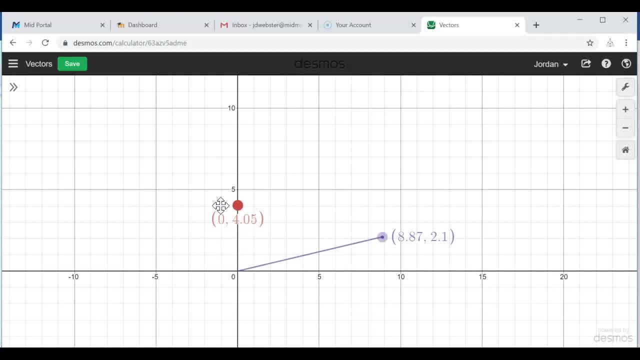 Dang it. Negative 1, 4 would be up here where my cursor is. I can't get the dot to move past the y-axis, but you can see that these kind of look close to orthogonal but they are not orthogonal, Obviously. 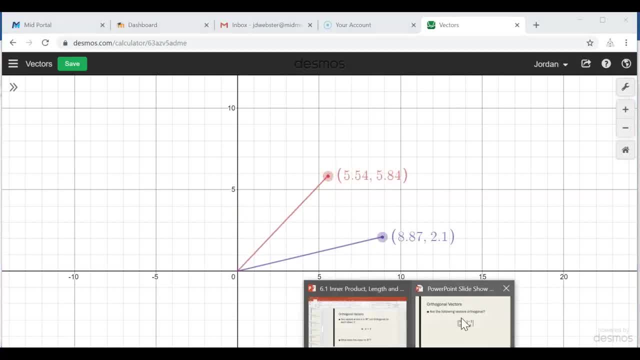 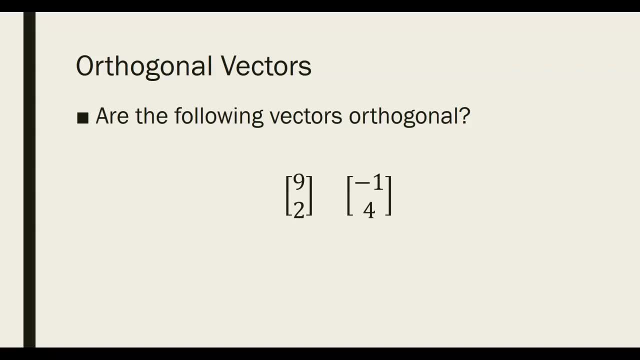 So there we go. So these are not orthogonal, While the previous example was orthogonal. I want you to test these two vectors and see if these two vectors are orthogonal. Alright, so hopefully you did that If you didn't push pause. So 2 times 4 gives me 8. 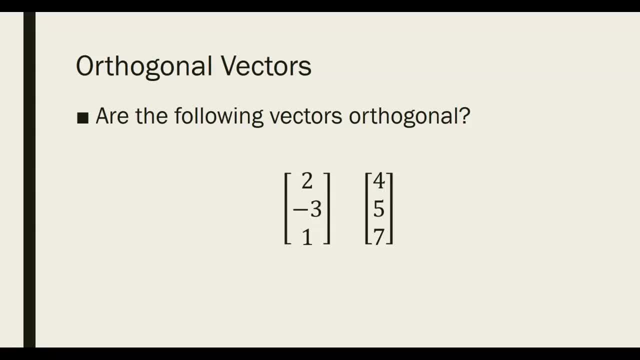 negative. 3 times 5 gives me negative 15. 2 times 7 gives me 7. so 2 times 4 gives me 8 minus. so 8 minus 15 plus 7 is the inner product of those two vectors and obviously that gives me out a 0. 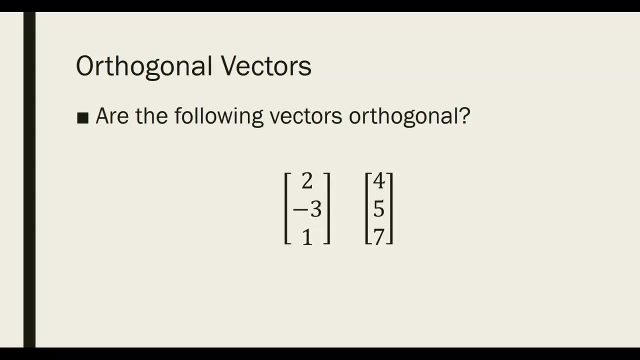 and therefore these two vectors are in fact orthogonal. Now one thing, one thing we get out of orthogonality is a Pythagorean theorem. Two vectors, u and v, are orthogonal if, and only if, they satisfy the Pythagorean theorem. Now, if you 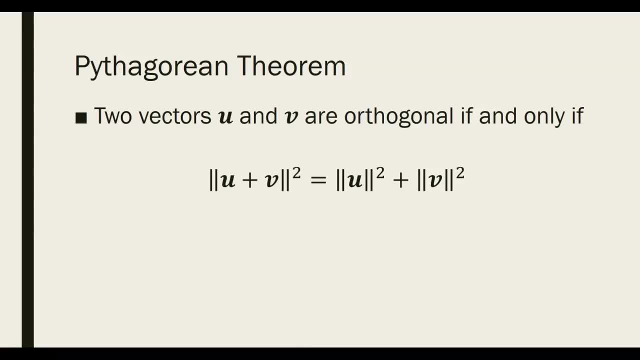 actually go ahead and do this. this is u plus v, orthogonal dot, inner product with another u plus v, And what you'll see is, if you expand this out, you get u squared plus u, dot, v plus v, dot, u plus v squared. Well, that's. 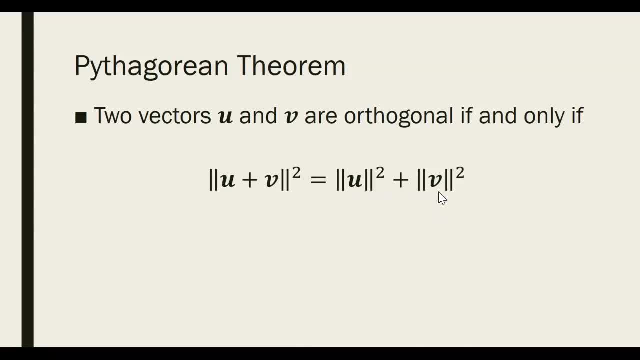 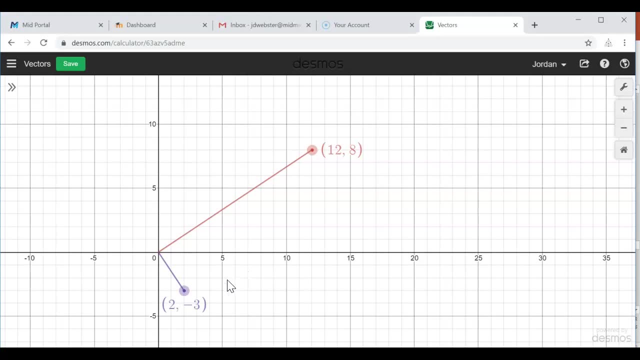 the same thing as these things if, and only if, the inner product is 0. So, again, Pythagorean. this is the Pythagorean theorem In two dimensions. what this would look like is the following: if we were to add two vectors now, by the way, 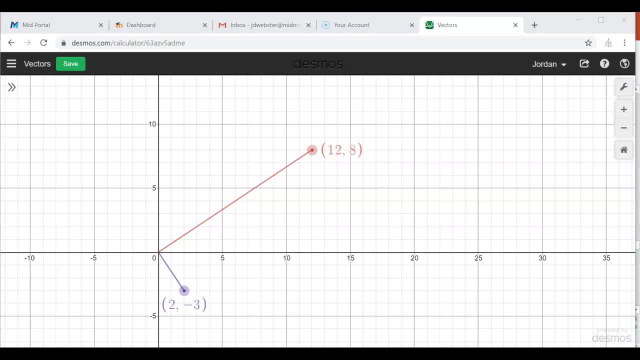 adding two vectors is not quite exactly what you think it is. So when we add two vectors, what I would do- let's say I wanted to add the purple vector to the red vector- what I would do is I would take this purple vector and try to 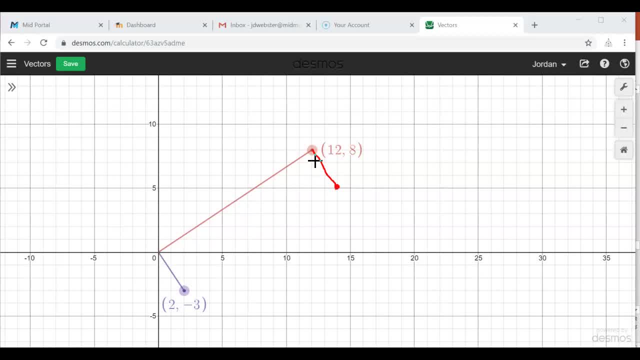 basically tack it all on to the red vector over here. okay, and when I add two vectors, I've created a third vector. I should have probably done that in a different, uh um, color, so let me erase that. so when you add two vectors, purple vector gets added. 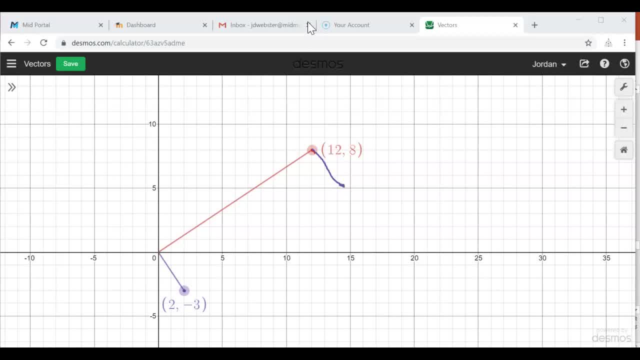 here. that creates a new vector that I've drawn in black. so this black vector is the sum, and you can see that this is going to form a right triangle. when the purple and red were orthogonal to begin with, okay, So we ended up with the length of the black vector. 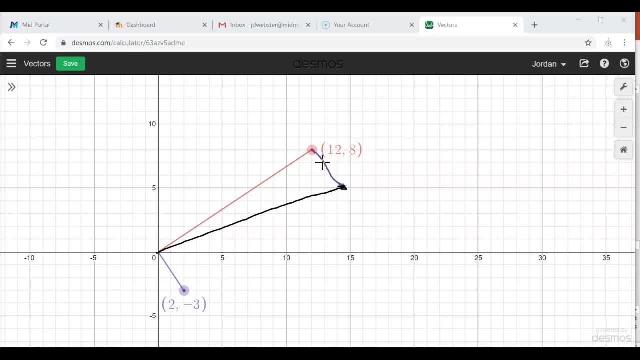 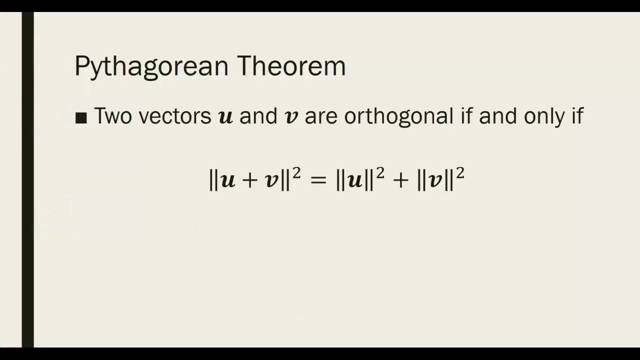 squared is length of the purple squared plus length of the red squared. okay, because of that right triangle. So there you go. that's the idea of that Pythagorean theorem using vectors. So this is the vector form of the Pythagorean theorem. We're not going to use that a whole lot. 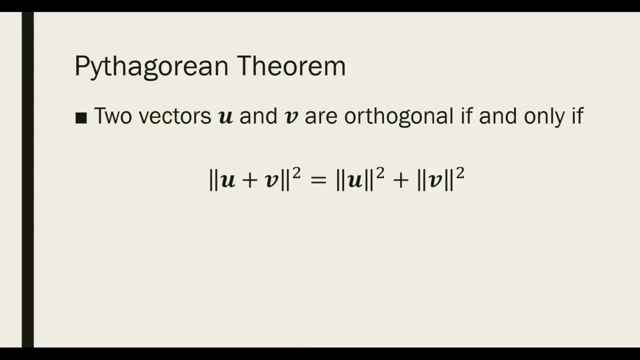 because it requires us to know when vectors are orthogonal. so that's not something that we deal with a whole lot in this class, but it is something that's nice to have seen once or twice. Now we have that two vectors are orthogonal or not. We can expand that. 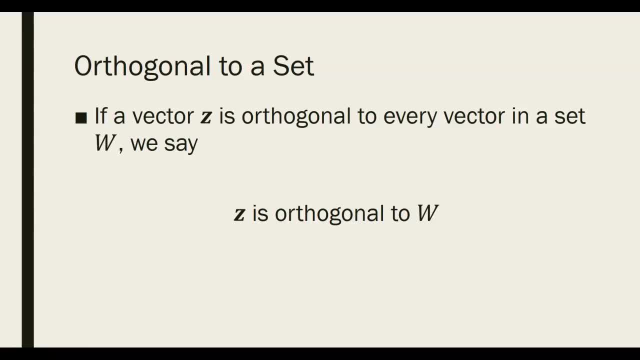 and say: a vector can be orthogonal to a set. Now a vector is going to be orthogonal to a set if the vector is orthogonal to every vector which is in that set. So if a vector is orthogonal to every single vector in the set, we say: 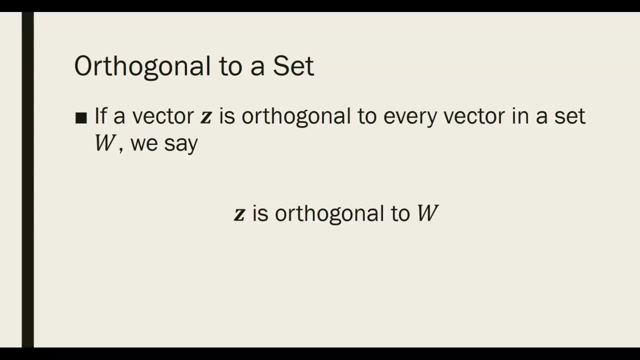 Z is orthogonal to that set. So let's take a look at this. I want you to try to calculate Z in our product with each one of these three vectors and determine if Z is orthogonal to the set W. Go ahead and push pause and see if that is true. 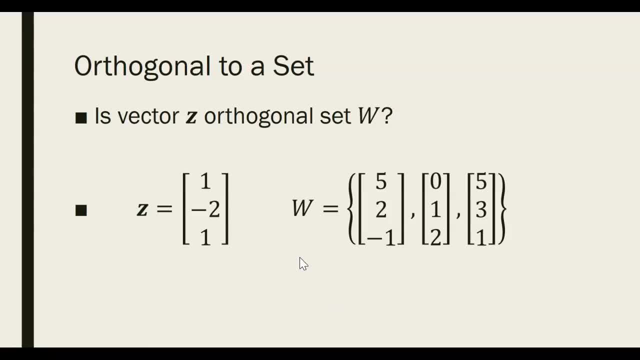 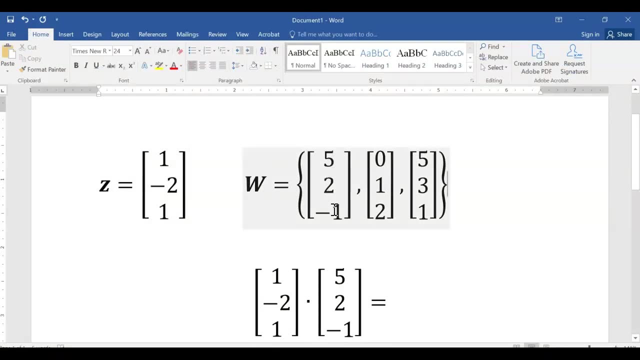 Alright, so let's go ahead and do that. Now there's three vectors in the set W, so I'm going to have to do three inner products. So I'm going to take Z and I'm going to take an inner product with Z, with this first. 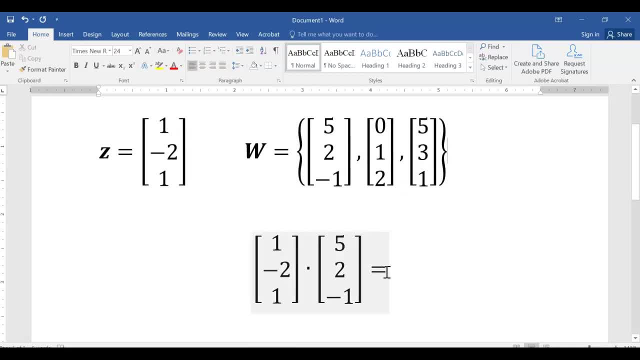 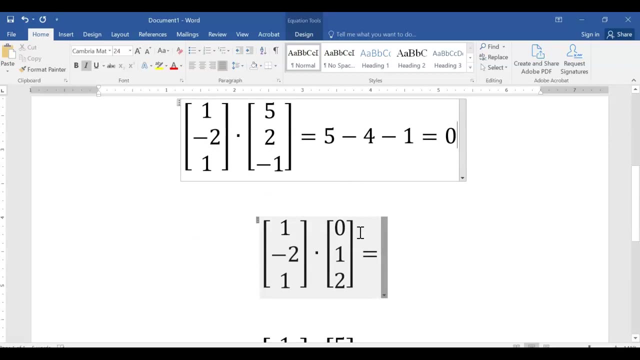 vector. So when I did that, I got 5 minus 4 minus 1, which is 0.. So that's good. Z is orthogonal to this first vector here. How about the second vector? Well, 1 times 0 is 0. 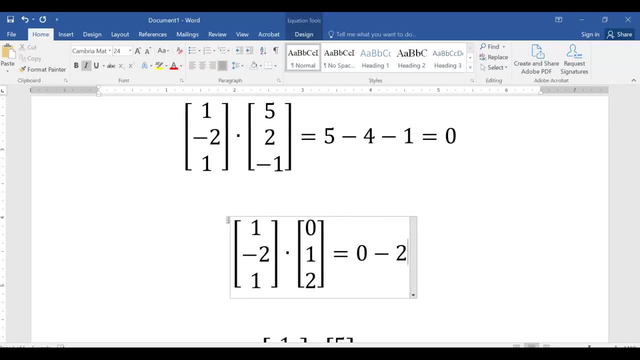 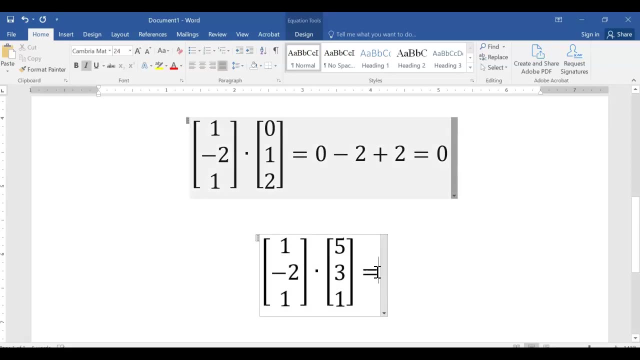 minus 2 times 1 is minus 2. plus 1 times 2 is 2, so I get a 0.. So good, Z is orthogonal to the second vector. Now let's take the inner product of Z with the third vector. 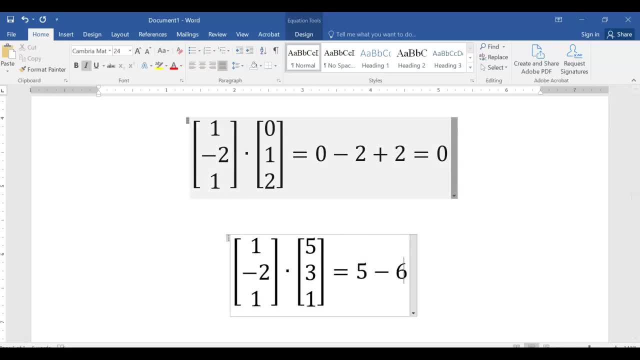 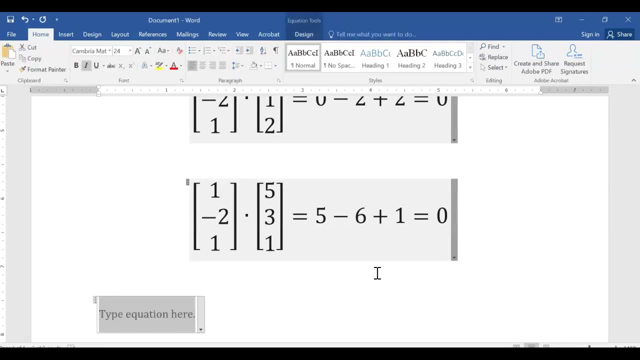 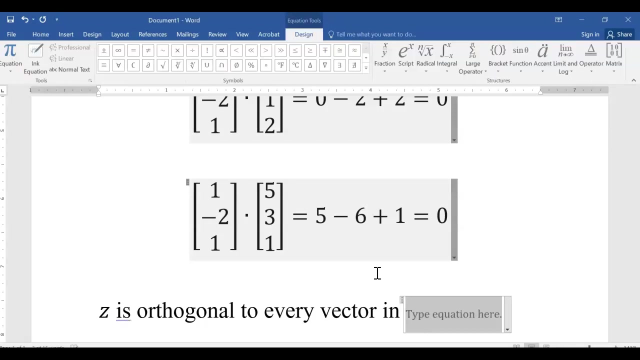 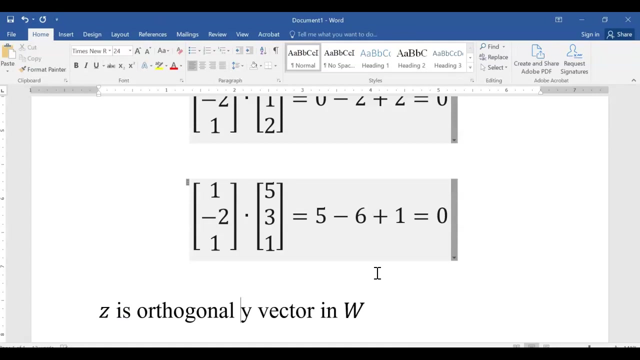 We end up with 5 minus 6 plus 1, which is also 0.. So Z is orthogonal- excuse me, is orthogonal to every vector in the set W and therefore we say Z is orthogonal to set W. Okay, Hopefully that all makes sense. 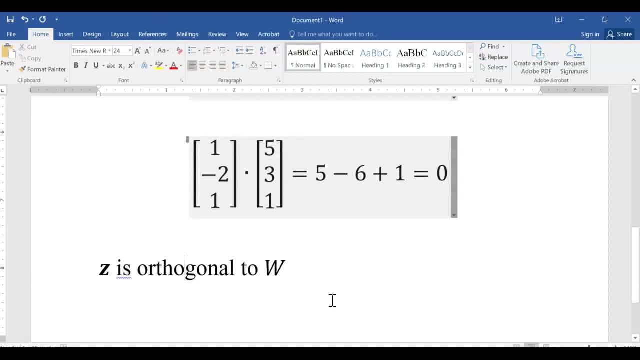 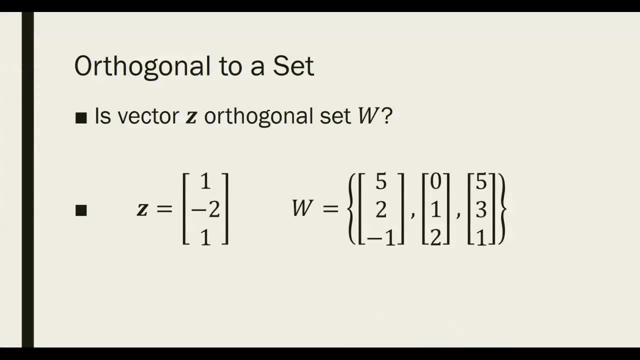 So if Z is orthogonal to every vector in the set, we say Z is orthogonal to the set itself. So I want you to try to calculate this. see if Z is orthogonal to W, given this Z and this W, Go ahead and push, pause and try to figure. 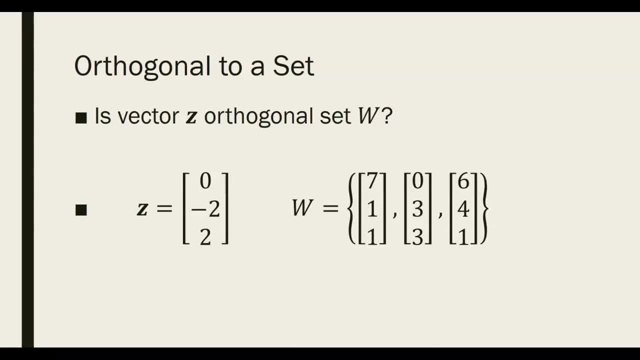 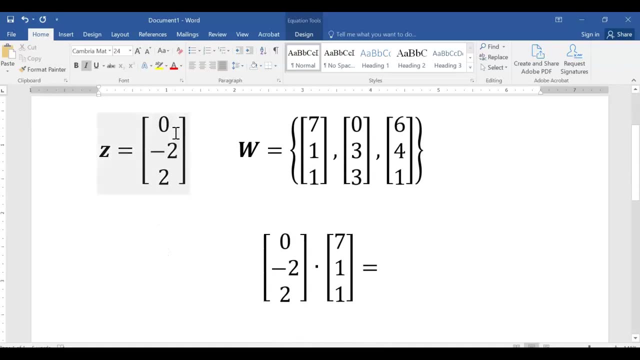 that out Alright, so hopefully you did that. I'm going to go through it. So take 0 negative 2, 2 times each vector in W. If I multiply 0 negative 2, 2 times 7, 1, 1, which is the first vector in W. 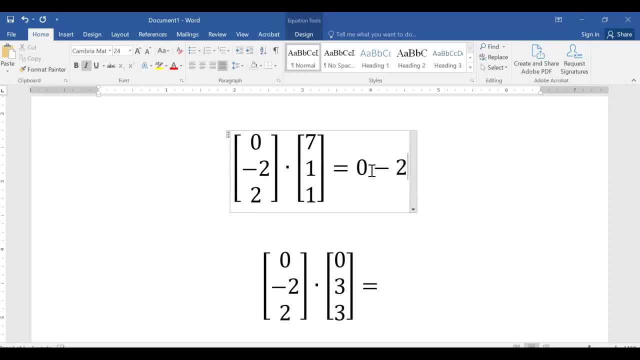 I get 0 minus 2 plus 2, which is 0.. Good, So Z is orthogonal to the first vector. When I take Z and do the inner product with the second vector, I get 0 minus 6 plus 6, which is 0. That's good. That means. 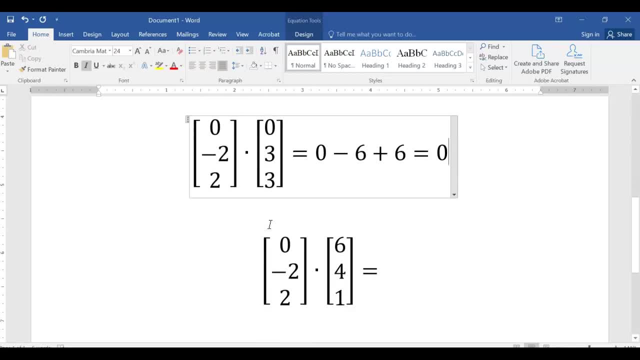 Z is orthogonal to the second vector And when I do the third vector I get 0 minus 8 plus 2, which is a negative 6. Z is not orthogonal to that third vector. Now, because Z is not orthogonal to that third vector, 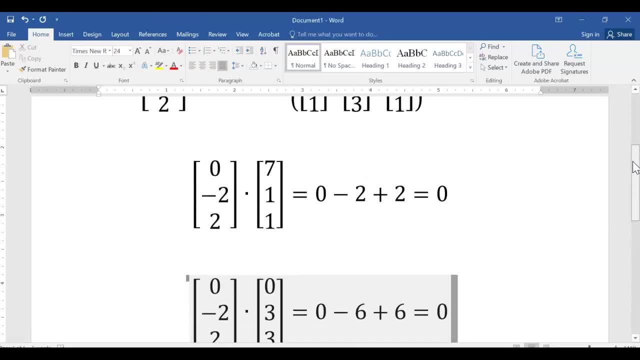 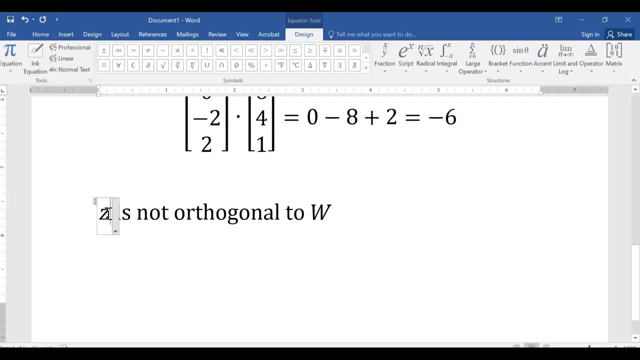 that means Z is not orthogonal to the set W. Alright, So if we were going to write this, we would say Z- oops is, let me do italics- is not orthogonal to W. Okay, So the vector Z is not orthogonal to W, to the set. 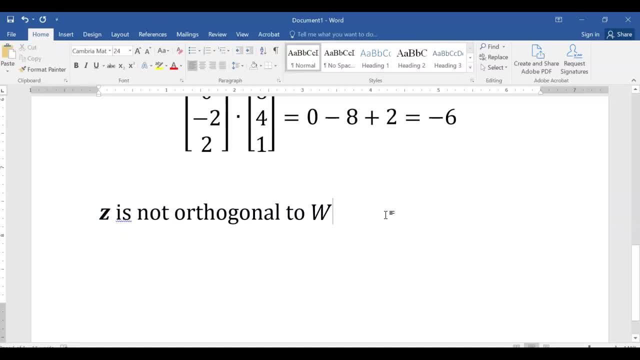 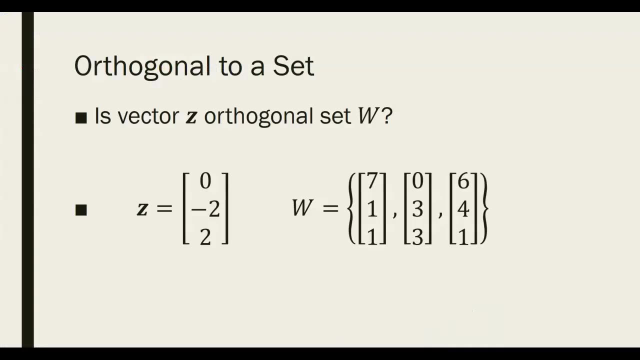 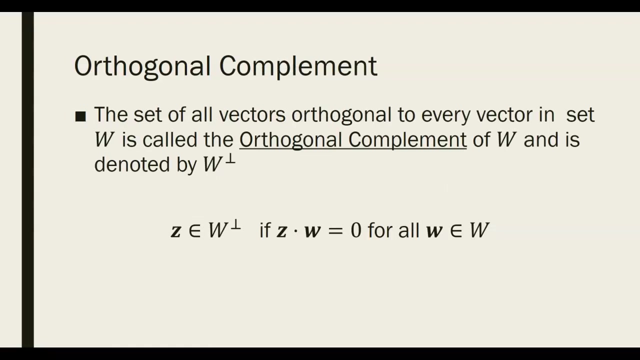 W. Okay, So it can be orthogonal to every single vector except for one. and if that's true, then it's still not orthogonal to the set. Alright, Now this leads to the idea of what's called an orthogonal complement. So we say that the set of all 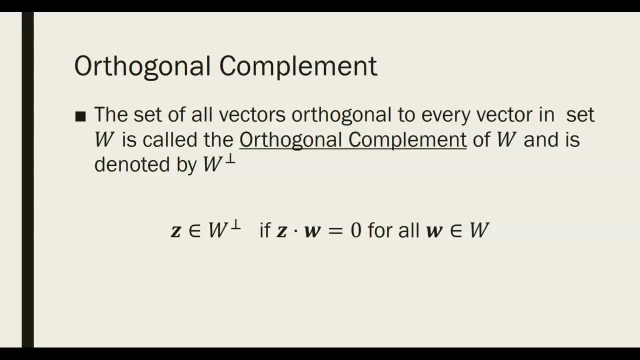 vectors orthogonal to every vector in the set. W is the orthogonal complement of W. Usually this is denoted with a W and then in for an exponent we put the perpendicular symbol. So orthogonal complement of W sometimes is- well, almost is always- written W with an exponent. 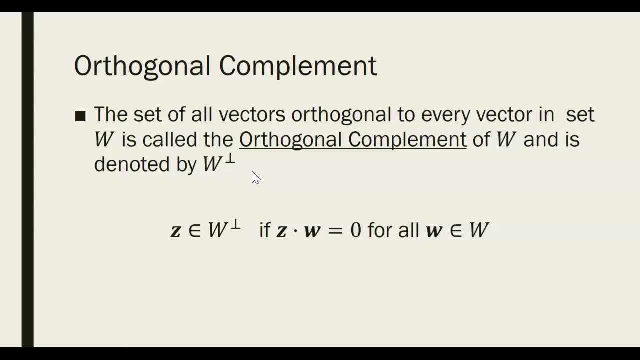 which looks like a perpendicular symbol. Okay, Which is again the upside down T. So in short, we have a vector. Z is in the orthogonal complement. if Z, when I take it, times the inner product of any vector from W, gives me out a zero. 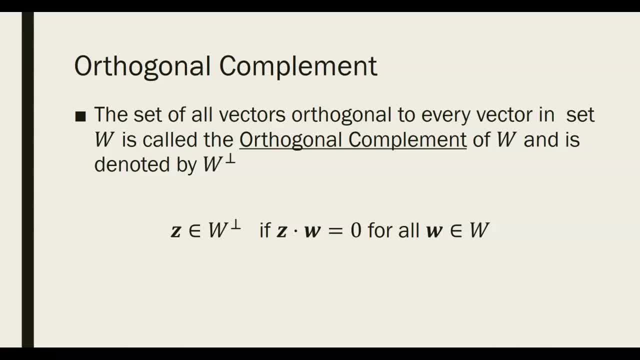 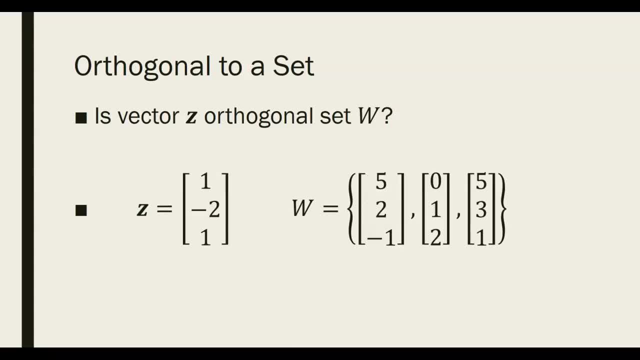 So we just need to if we're going to check if Z is in the orthogonal complement. that is checking what we just did. So, for instance, in my, when I looked at orthogonal to a set two slides ago, we saw that Z was orthogonal to every vector in W. 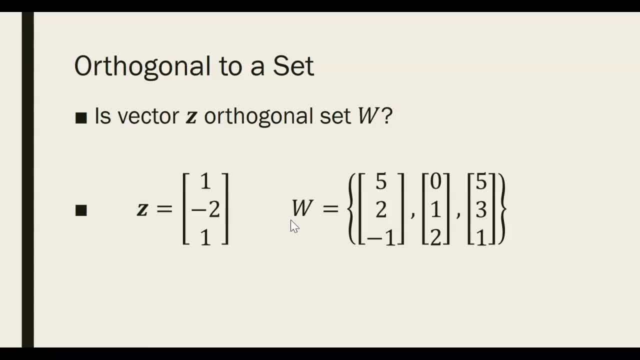 So we would have said Z is in the orthogonal complement of W, This Z, because when we took the inner product of this Z with the last vector in the set we didn't get zero. So this Z is not in the orthogonal complement, This Z is in the orthogonal complement. 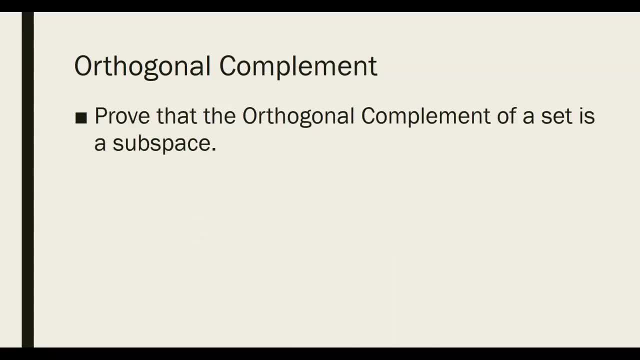 of W. Now it turns out that the orthogonal complement of a set is in fact, a subspace. So we're going to take a look at that. We're going to prove that the orthogonal complement of any set is a subspace. Now, hopefully you remember. 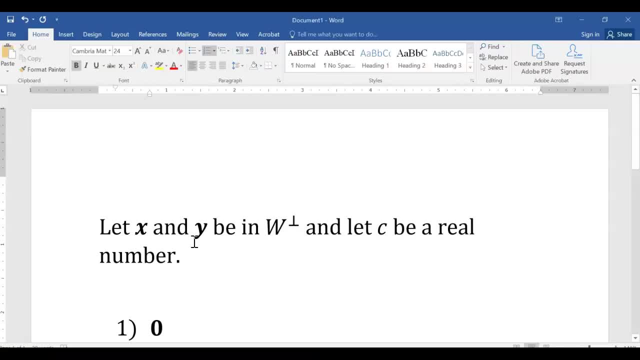 the three properties of being a subspace. So to be a subspace, we have to have the zero vector, we have to have closed under addition and we have to have closed under scalar multiplication. So we're going to let two vectors, which we call X and Y, 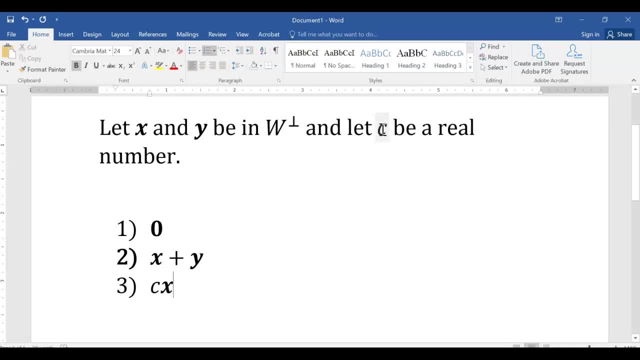 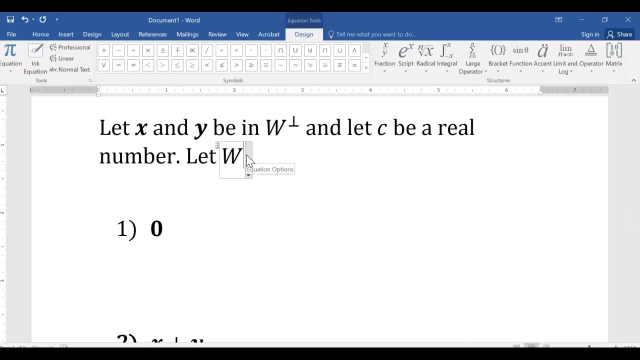 be in the orthogonal complement and we're going to let C be some real number. So, first off, let's focus on zero. Okay, Is zero in the orthogonal complement. Well, let's let W, as in lower case W, be a vector which is in. 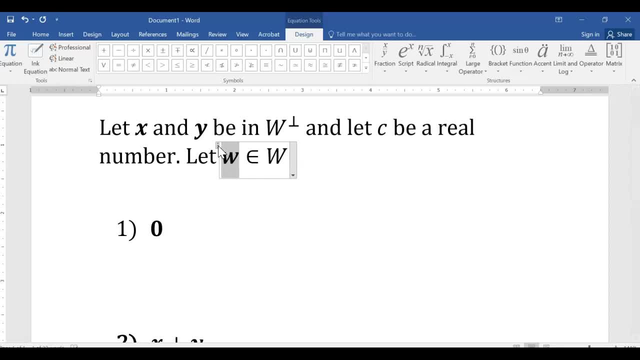 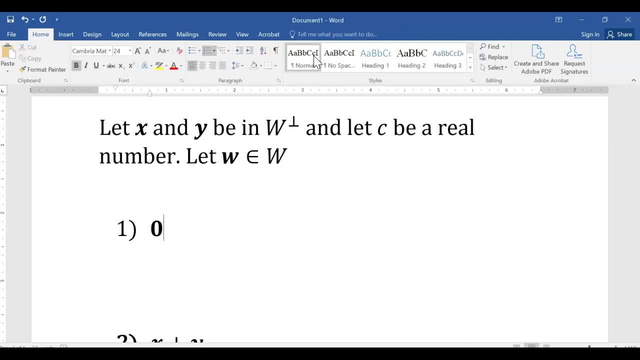 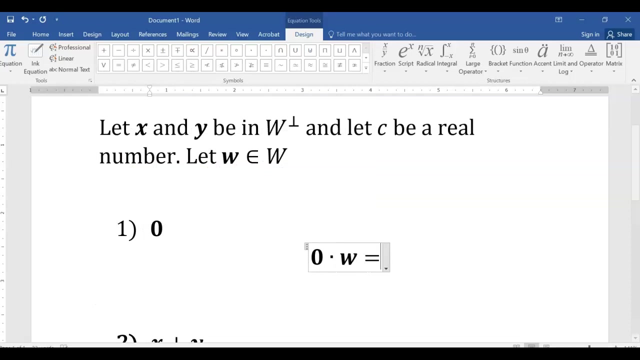 the set W. It can be any vector in the set W. Well, if I take- oops, yeah, that's what I was looking for- if I take the zero vector and I do an inner product with any W in my set W, well, zero vector inner product. 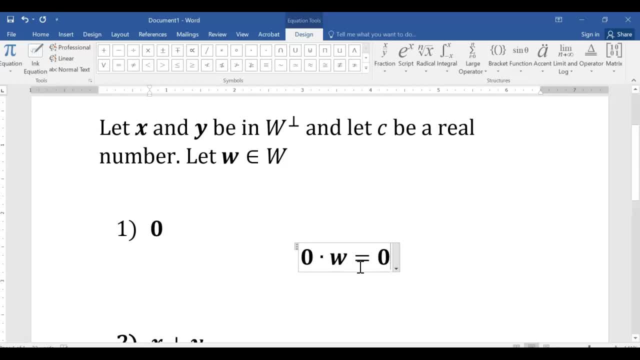 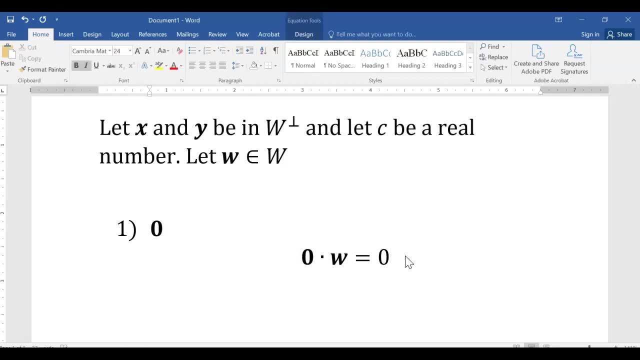 with anything, is going to give you out the real number zero. So what this means is that, yes, when you take the zero vector, it is going to be orthogonal to everything. every vector in W- Okay, So zero vector- it must be in the orthogonal complement. 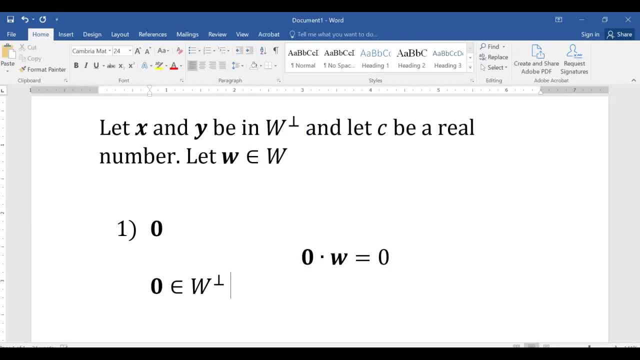 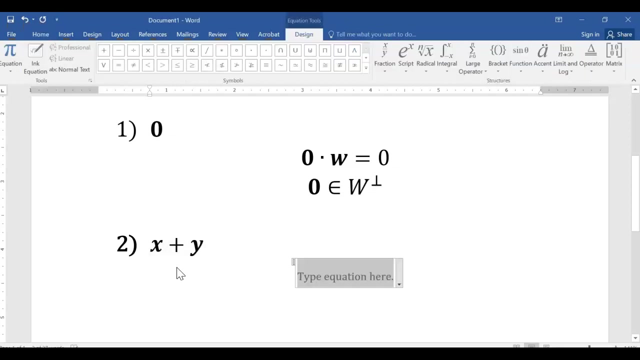 of W. Alright, There you go. So zero vector is there. What about closed under addition? So let's take the vector x plus y, excuse me, and let's dot product that with the vector W. Now, because of the rules of inner product. 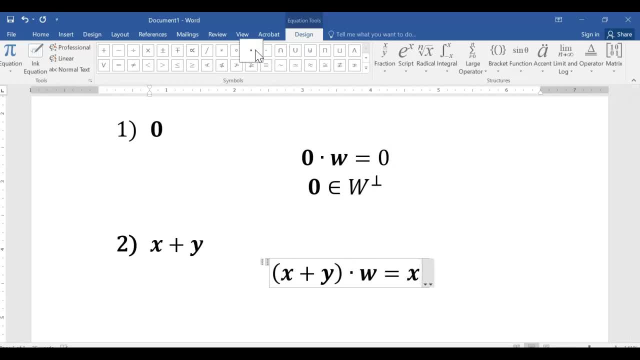 we're going to get x, inner product W. by the way, I've mentioned this a couple of times- inner product is always symbolized with a dot, so sometimes people call this the dot product As well. So because of the way that the inner product or the dot product, 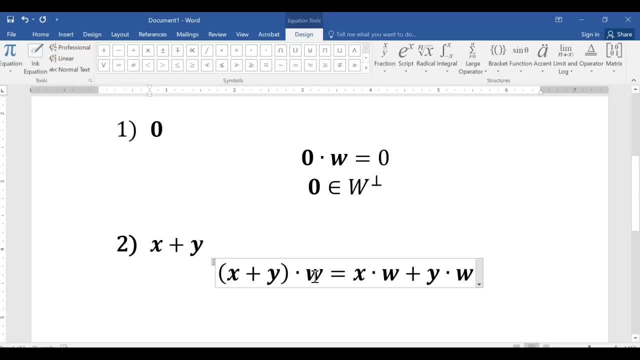 distributes over addition. we can distribute and say x dot W plus y dot W. Now remember x and y individually were already in the orthogonal complement, meaning that x dot anything in W is going to give me the zero vector, y dot anything in W is also going to give me the zero vector. 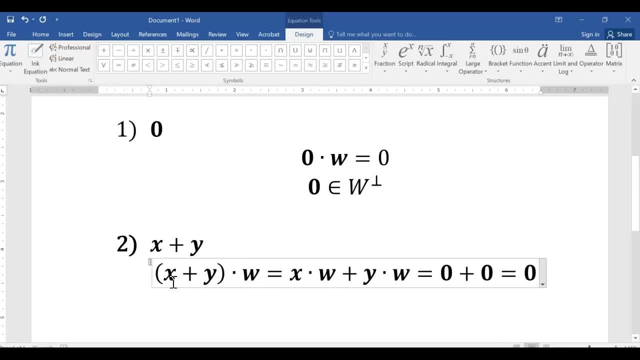 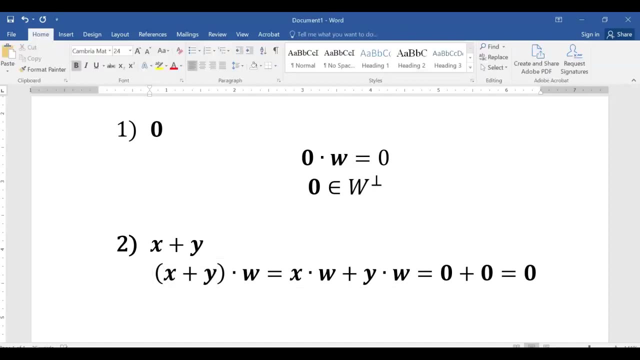 and so what we see is that when you add two vectors which are in the orthogonal complement, that sum is also going to be in the orthogonal complement. So there we go. So the sum of x plus y is in the orthogonal complement. therefore it's closed. 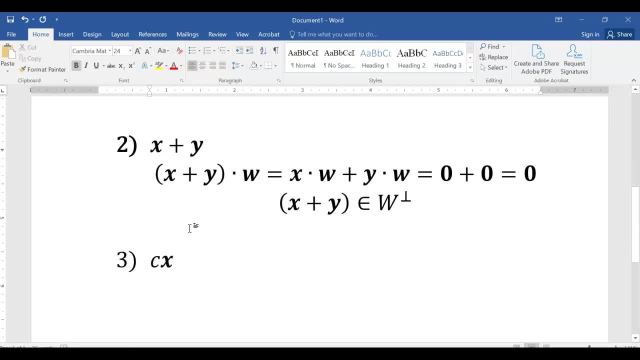 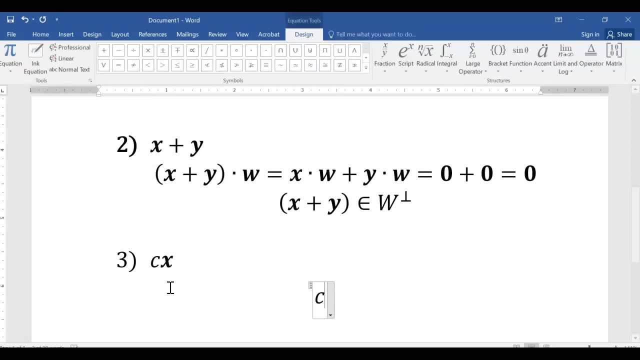 under addition. Now, as far as scalar multiplication goes, we're going to do a very similar thing. 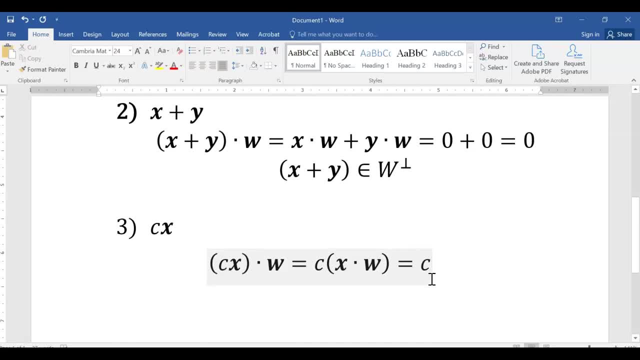 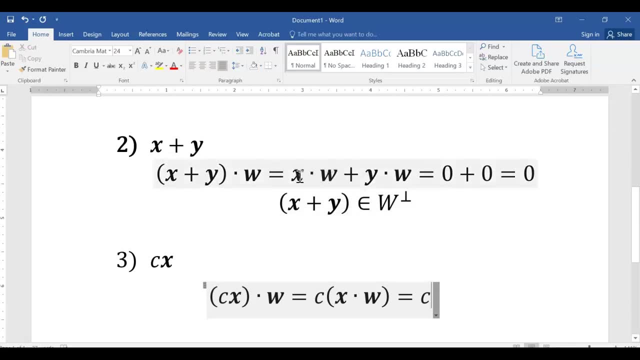 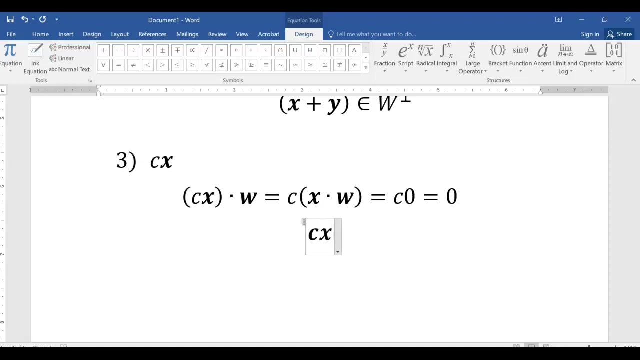 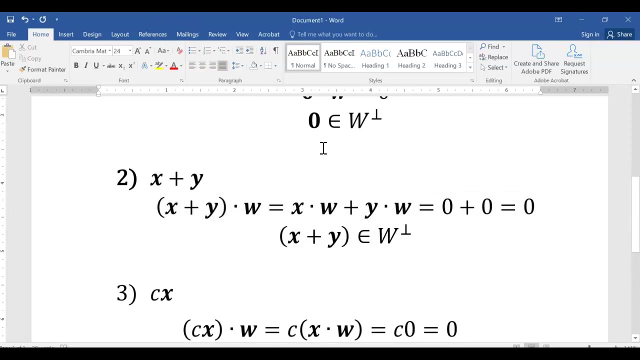 What we're saying is that the zero vector is in the orthogonal complement. The orthogonal complement is closed under vector addition. 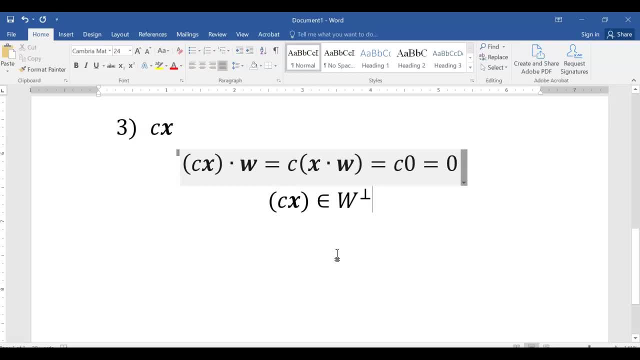 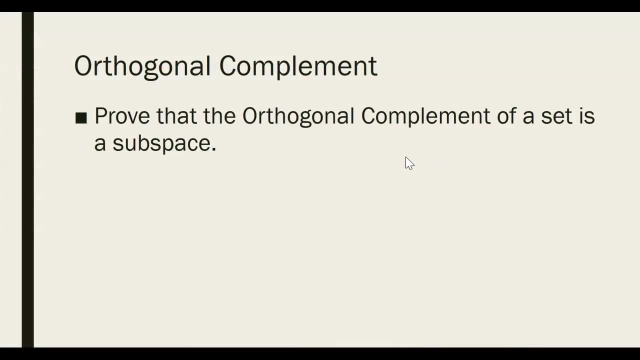 The orthogonal complement is closed under scalar multiplication. So therefore, the orthogonal complement is, in fact, a subspace of whatever vector space I'm dealing with. So what I would like you to do is ask yourself: is z in the orthogonal complement of w? 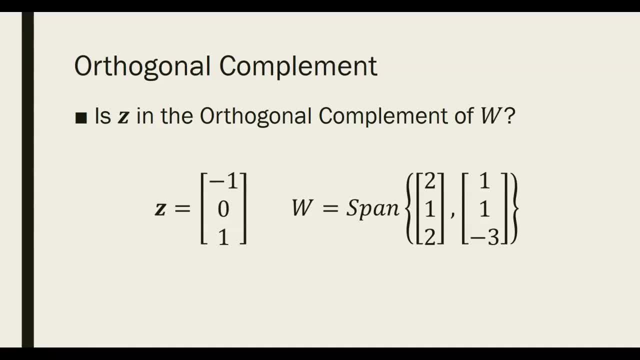 And w is going to be the span of those two vectors. So push, pause and go think through if z is in the orthogonal complement of w. Now there's going to be a couple of ways we see this, But let me start out with saying this: 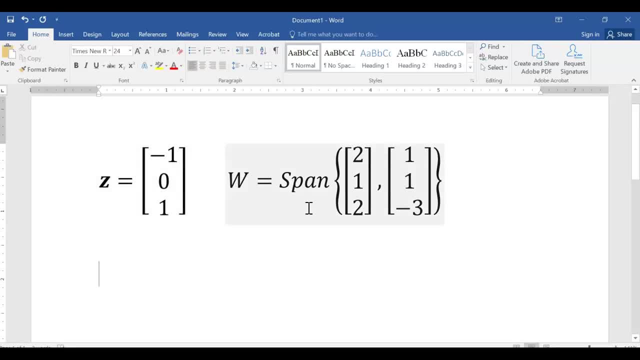 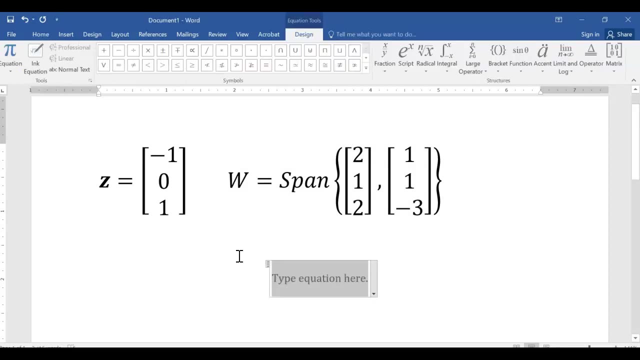 Now z is this vector here, negative, 1,, 0,, 1.. And w is the span of this. So we have infinitely many vectors in w, But we can take care of them all at once if we realize that any vector in w can be just written as a coefficient. 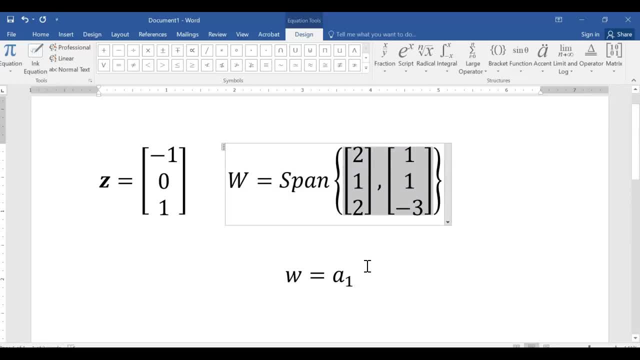 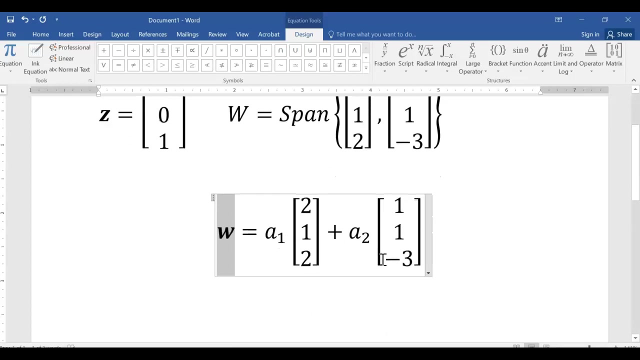 times the vector 2, 1, 2, plus some other coefficient times the vector 1, 1, negative 3.. So any vector that's in w is going to be written as a linear combination of these two vectors: 1, 2 and 1, 1, negative 3.. 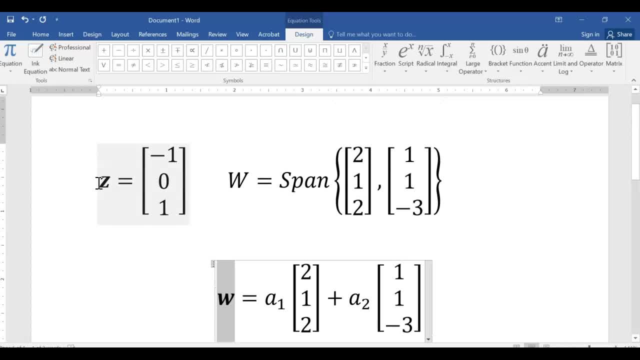 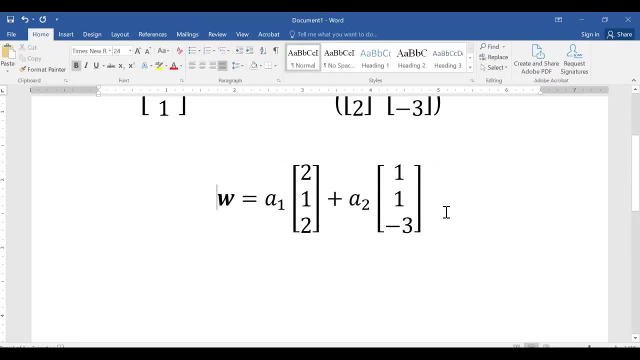 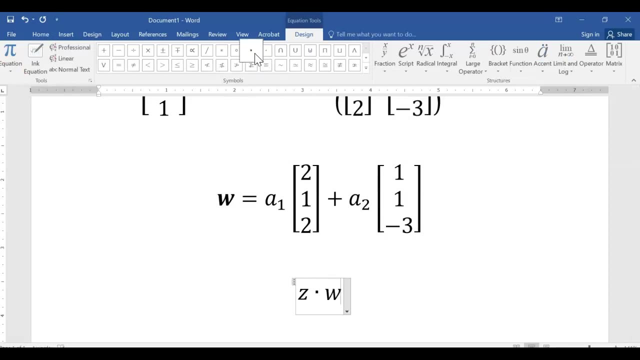 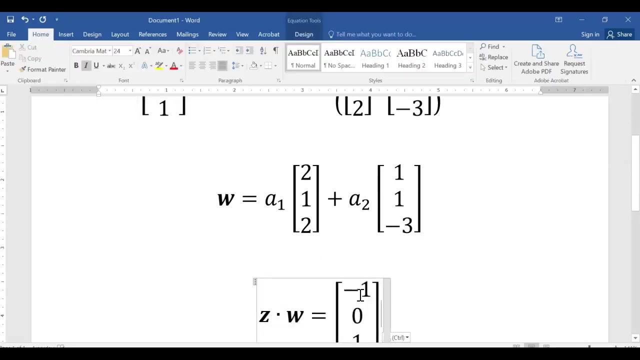 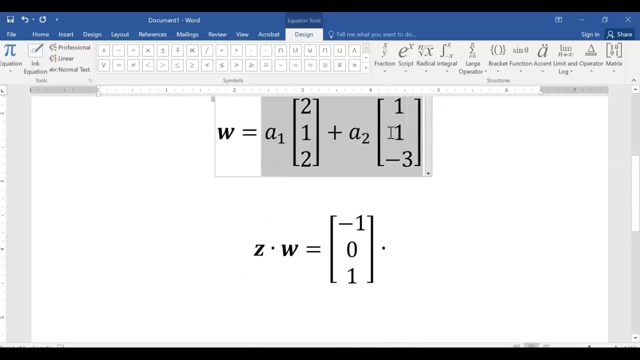 So all we have to do is take the inner product of z times some arbitrary w. Now, hopefully, what we see when we do that- z inner product and arbitrary w- is that I'm going to take this vector inner product with the linear combination. 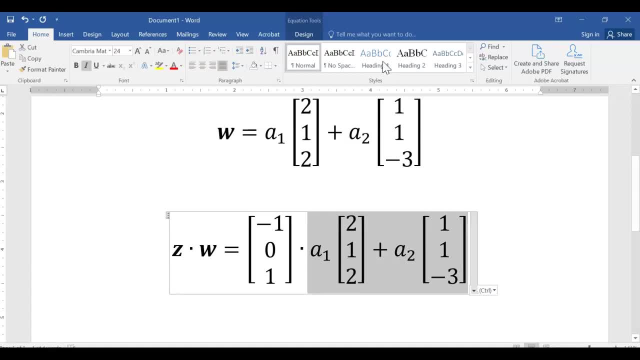 By the way, the linear combination. I should probably put that. hopefully I can put that in parentheses. There we go, And what's going to happen? Well, using the same distributive property that we did before, I can take and set. 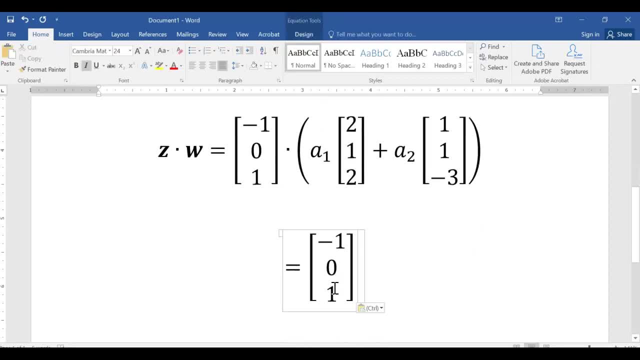 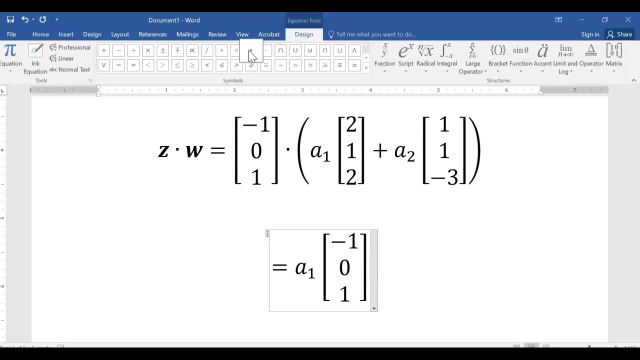 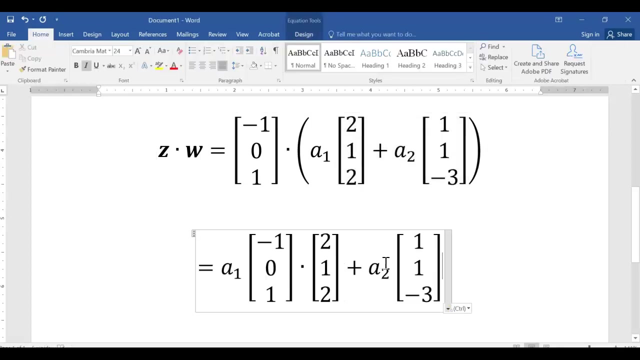 negative 1, 0, 1 inner product with 2, 1,, 2, and I can factor out an a1 in front of that, And then the same thing goes. I can take negative 1, 0, 1,. 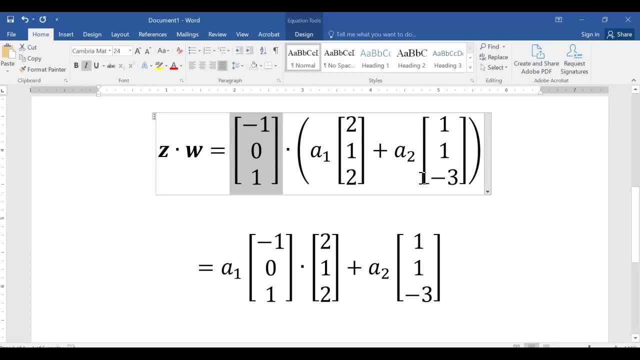 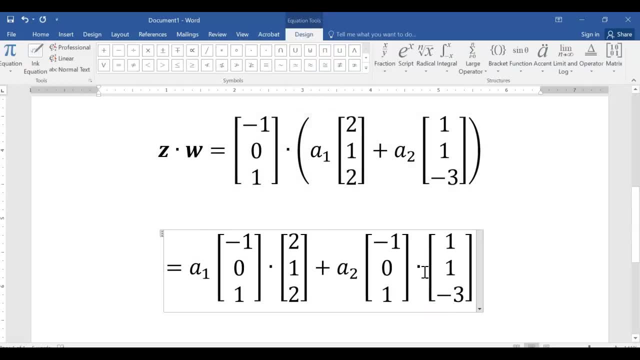 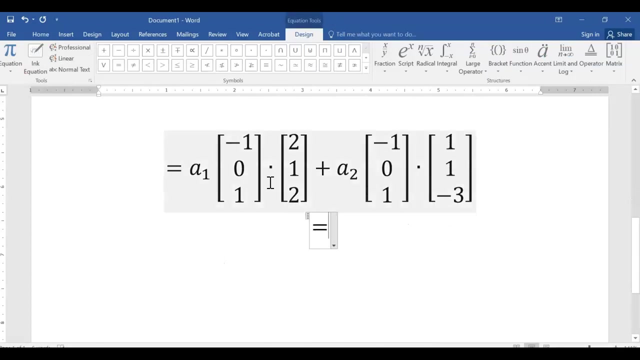 distribute it in here and factor out an a2.. Make sure we have our inner product or our dot product there. And what we see is: well, when I take this first dot product, we get negative 2,, 0,, positive 2.. 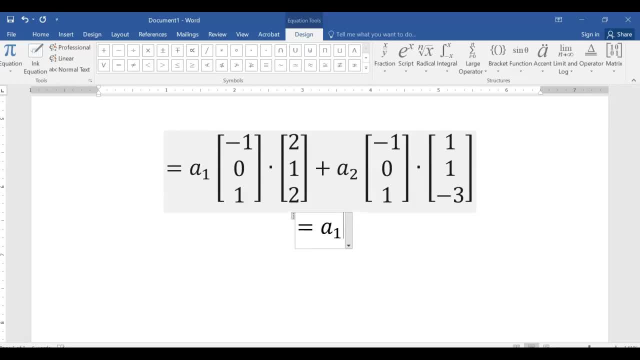 So you get a 0.. So you get a1. Times 0, that's the real number, 0.. Plus a2.. Here we get negative 1, 0,, negative 3.. So times a negative 4.. 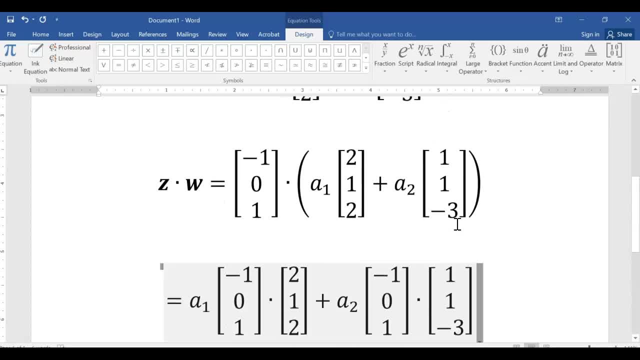 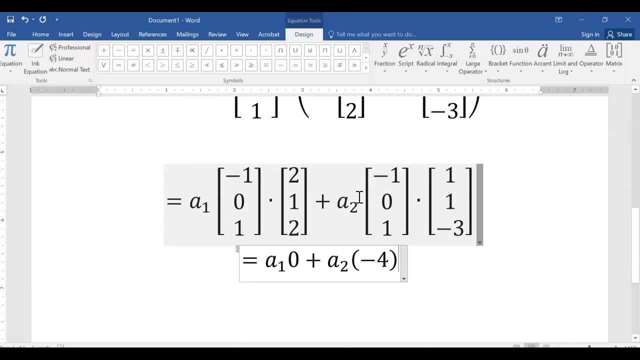 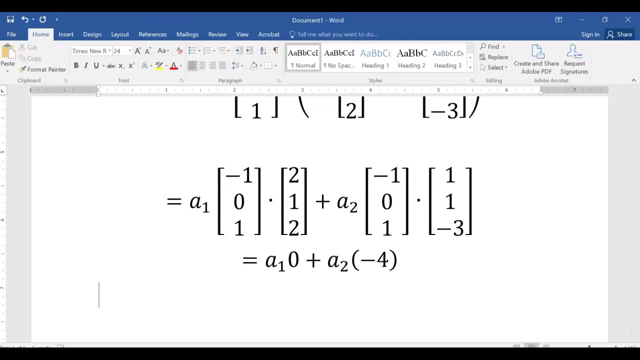 So what we can see is that there are values, for a2 in particular, In which I don't get out a 0 when I inner product it, So this can be non-zero. In fact, negative 4a2 is often non-zero. 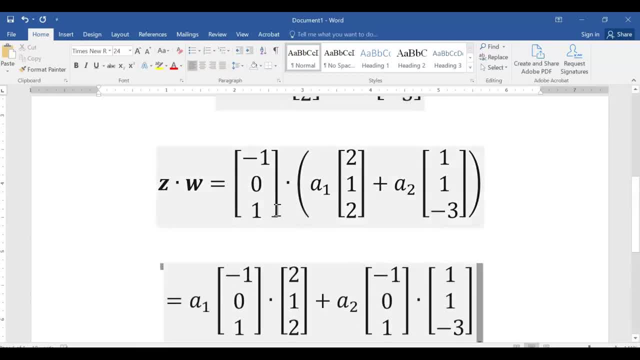 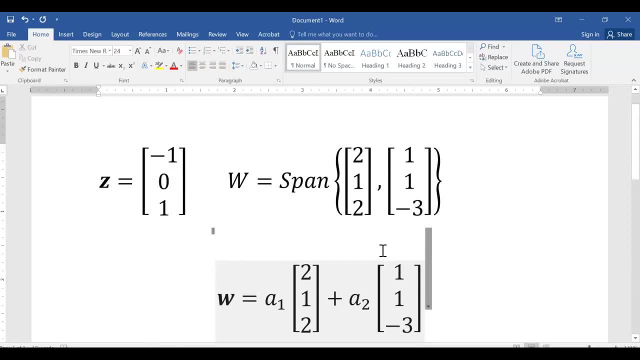 All right, So we can find vectors in w where z is not orthogonal to those vectors in w. All right, So z is not in the orthogonal complement of w. Now this was kind of a lot of work to write every w as an arbitrary vector. 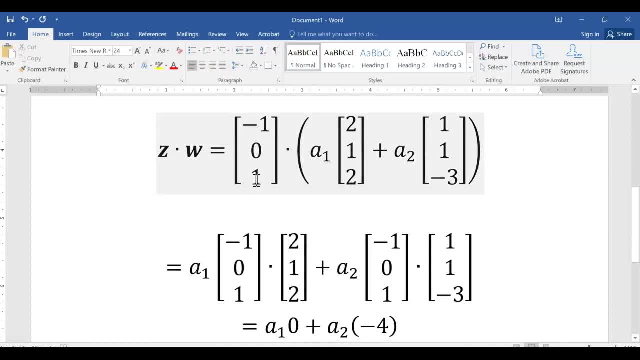 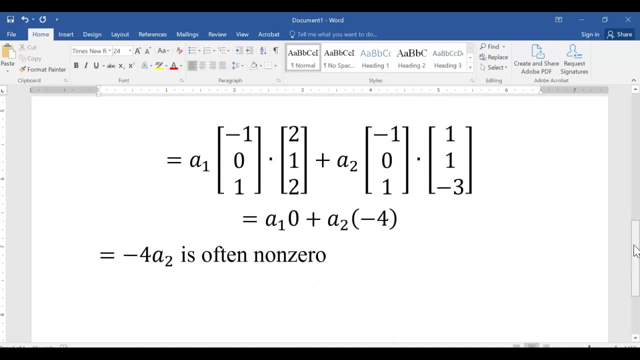 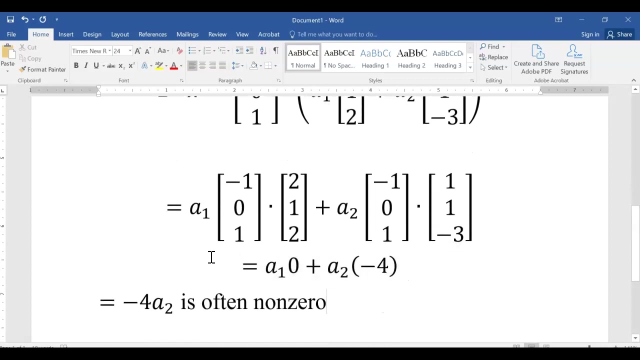 Really, what's this hinge on? This hinge is on the fact: is z orthogonal to every element in a basis for w, Or at least is z orthogonal to every vector in a spanning set for w. In this case, z was orthogonal to one element in my basis. 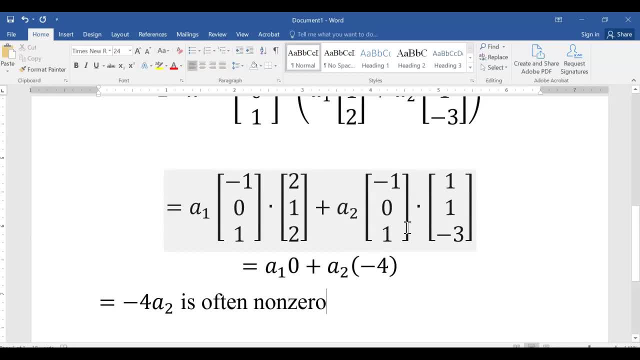 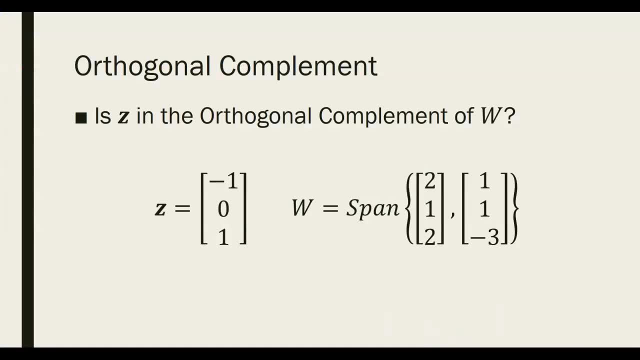 but it was not orthogonal to the other. Therefore, z is not orthogonal to the set w itself. I would like you to check and see if z is in the orthogonal complement of this set. w Go ahead, push pause on the video and do that. 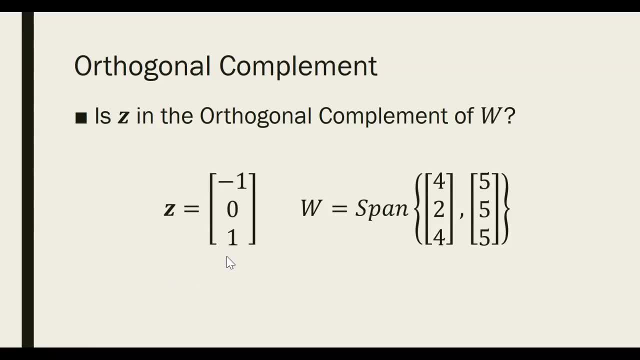 All right. So, again, knowing that all we have to do is check to see if z is orthogonal to the spanning set, All we really need to do is check if z is orthogonal to 4,, 2,, 4, and if it's orthogonal to 5,, 5,, 5.. 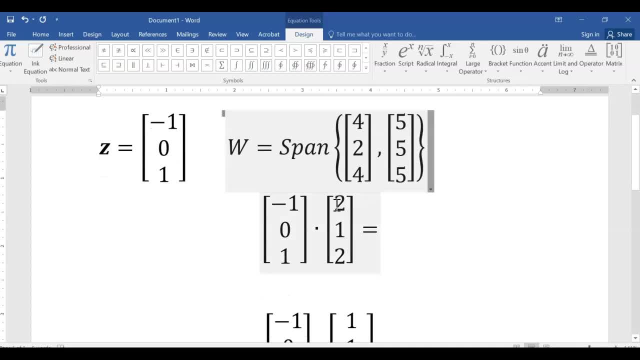 So we take our z. We look at the inner product of 4, 2, 4. with z You get a negative 4 plus 0 plus positive 4. That gives you 0. So z is orthogonal to 4, 2, 4.. 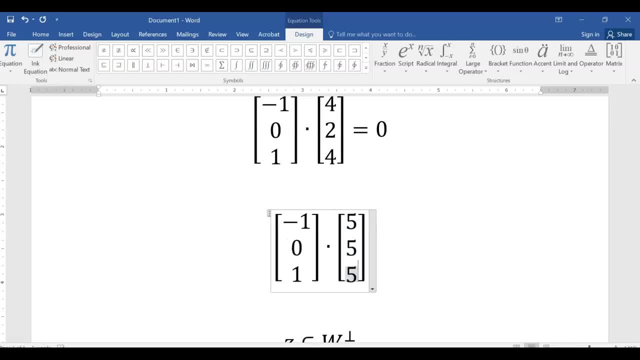 And then we check to see if z is orthogonal to 5, 5, 5.. In this case we're going to get negative 5, 0, positive 5.. When you add those up, you get a 0. 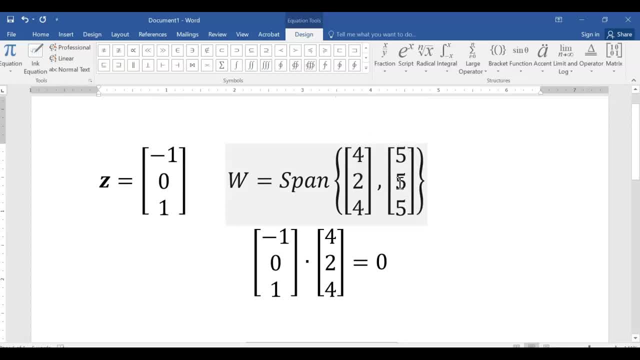 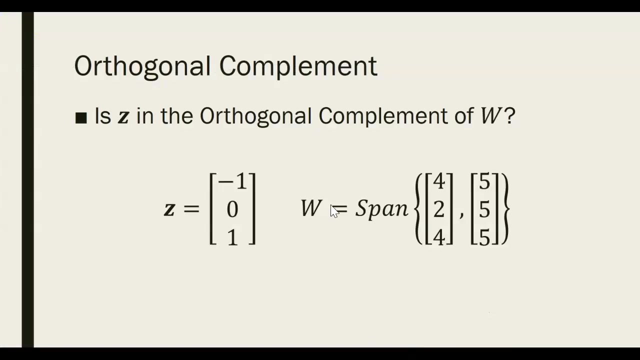 So z is orthogonal to both these two vectors And therefore z must be orthogonal to the span of those two vectors. So z is orthogonal to every single vector in set W. In other words z is in the orthogonal complement of W. So when we deal with sets, 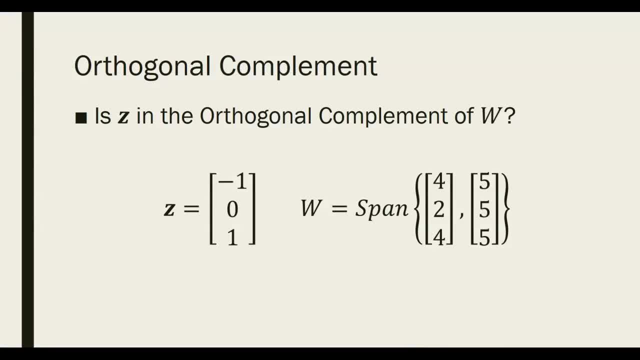 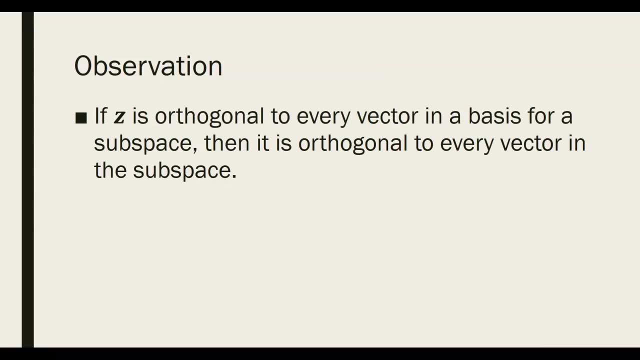 which are of infinite size, then we're looking for a basis or a spanning set for that set, W, And this is the observation we were going off of. If I have a vector z that is orthogonal to every vector in a basis for a subspace, 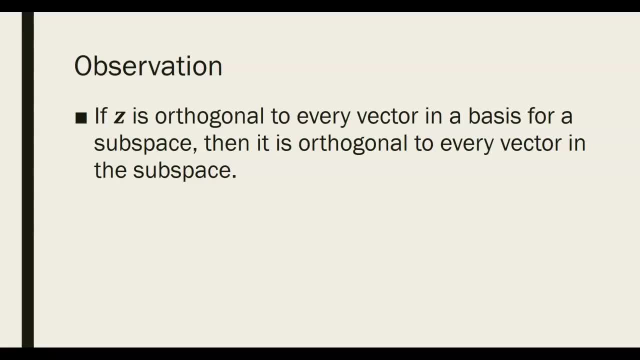 then it must be also orthogonal to every vector in the subspace itself. All right, So we looked at a lot of things. We're going to deal with a lot of orthogonality in the coming sections, But again, all of this hinges off. 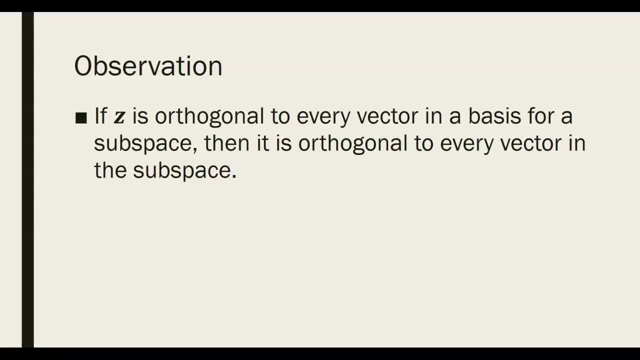 of inner products, the concepts of vectors, inner products, length and then orthogonality. We'll do some more work with orthogonality again in the next few sections, So make sure you're on top of knowing what's going on. 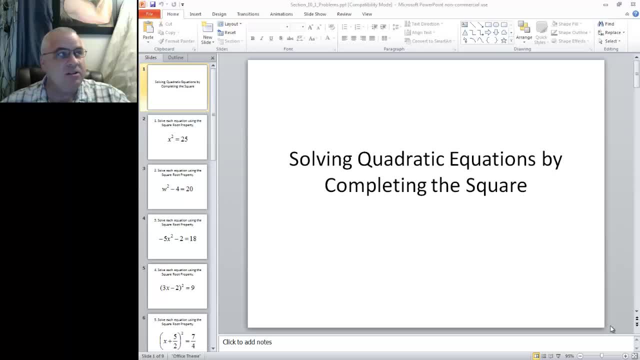 Let's take a look at solving quadratic equations by completing a square. The first topic we're going to take a look at is square root property. I don't see my tablet up and running, so I guess that's my first step is get the tablet. 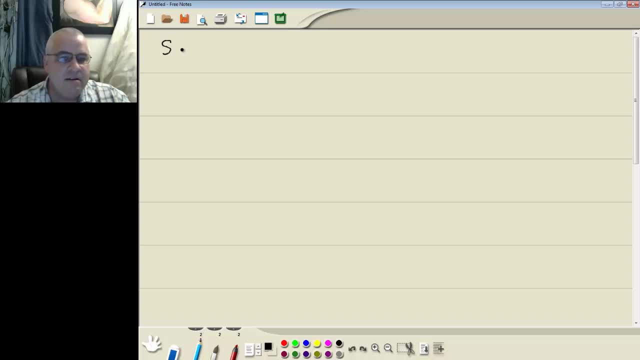 There we go: Square root property. Square root property says: if you got something squared equal to something else, then you got to draw up a squared and you put a plus or minus square root around the other side. Now that's pretty vague if you got something squared equal to something else, but it really.